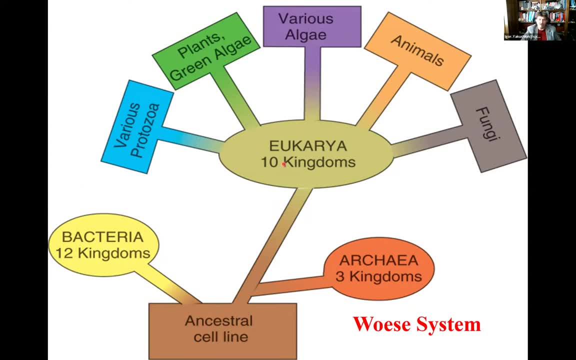 We already talked about several. I told you we have like four major kingdoms And we already Pretista as well. The algaes are kind of combined together. That's why, for then, there is a plant- animals and fungi. As a matter of fact, this week we'll start on the plants. 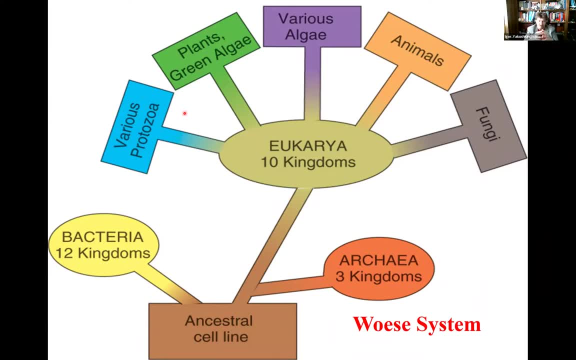 So, but the pretista is a kind of collecting group. Remember, I was telling you that if it's not 100 percent plant, animal or fungi, it goes right now into that particular group known as the pretista. That's one of those particular tree of life. 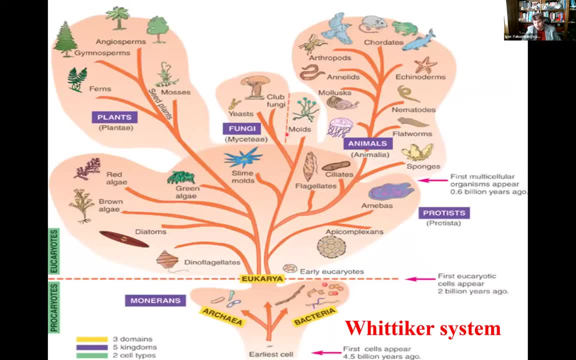 There is a little bit more Detailed one, but once again early cell, somewhere around four point five, probably closer, but maybe four point five, four point two, billions of years basically. as soon as Earth's cool off enough- well, basically, to like about 100 degrees Fahrenheit on the surface, we start seeing the presence of life and then start diversifying. 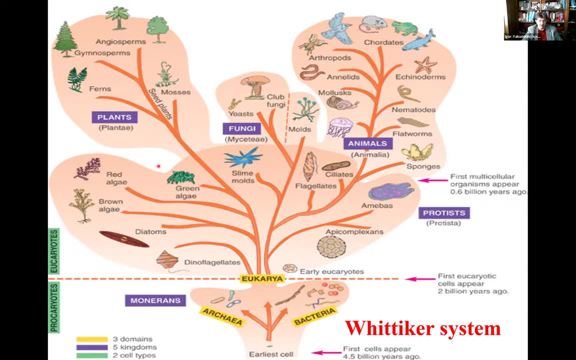 And you can see the bunch of different projects. We've got a lot of plants, we've got a lot of plants, we've got a lot of plant owners that are doing work, And the other part of the art is sort of you seeing what is today. 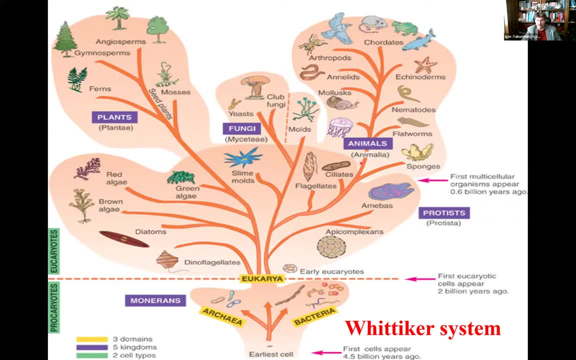 We'll call this weekend, a couple of next couple of weeks. We'll talk about the seedless plants, seeded plants of flower plants, all that particular stuff, And then we already talk about the fungi, And then we'll talk about the animals. 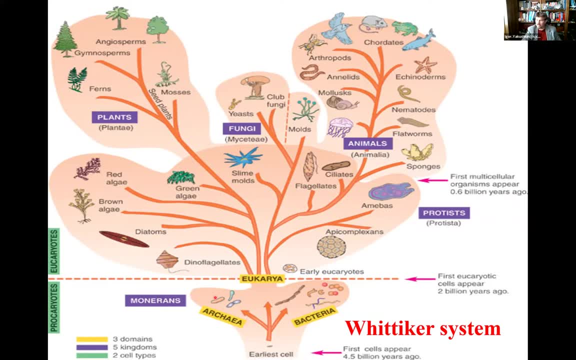 prokaryotes and eukarya, pretty much everything else. there was several students who still believe that if it's a single cell, organelle, uh organism, like a protist, like a euglena or diatom or amoeba, it's a eukaryote, it's a prokaryotic organism. no, they're not prokaryotes, they're actually eukaryotes. 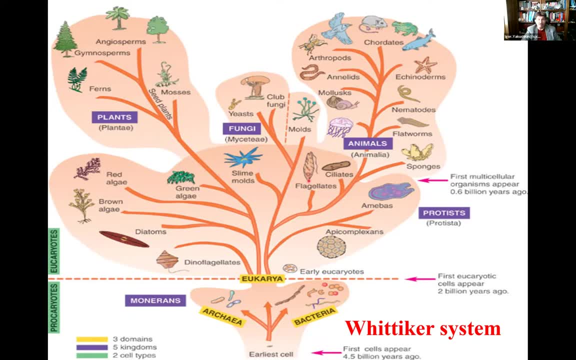 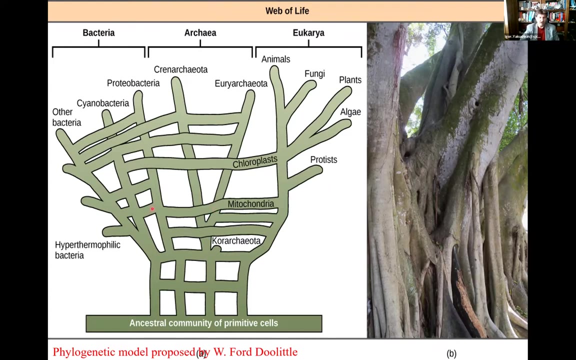 they have the uh nucleus and membrane bound organelles, so they are quite complex. that's the answer on the short, uh, short answer. and then there is another very interesting thing which shows pretty much the same tree, but now we have the cross-section, something which known as the 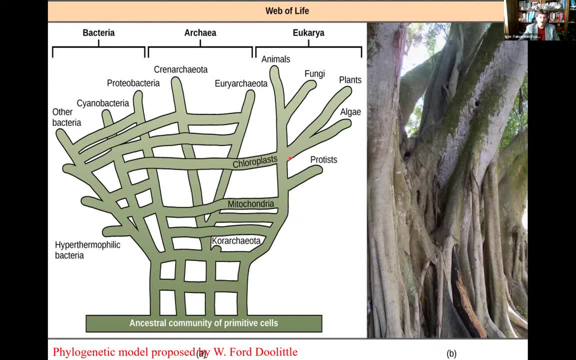 interspecies or intergroup uh. moving off the uh of the genes, dna from bacteria has been embedded into some of the animals. interesting, some of the fungi plants. you probably heard about genetically modified organisms, right, gmo, bad, we don't really know. we actually uh are the like guinea pigs for the genetically modified uh produce. 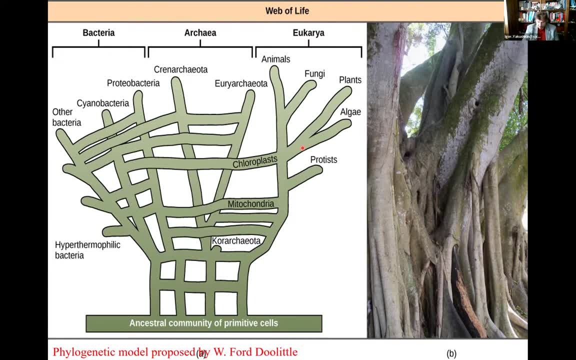 we don't know the long term of the gmo, so but it happens in the nature. now we are copying the nature and we can take the gene from, let's say, flounder and stick it into the potato. you can say: why do we need to take the flounder or shellfish and stick it into a potato or tomato? well, 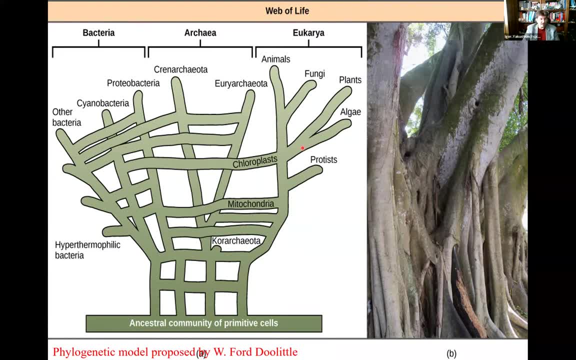 apparently it will not make. well, it will make those particular genetically modified organisms- potatoes and tomatoes- bad tasted for the pests. pests will avoid that, like we are tasting potato away. but it actually happened. now we're doing it artificially, but it happened on multiple occasions- horizontal gene transfer, so to speak, from one group to another, such as chloroplasts, remember. 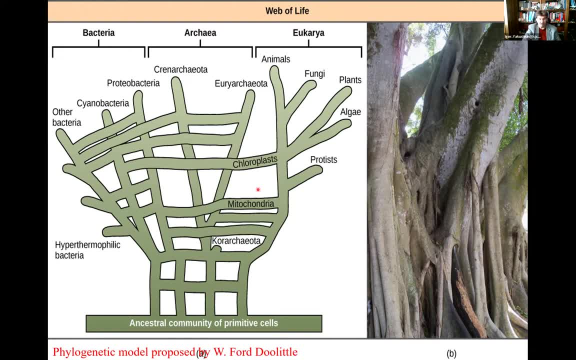 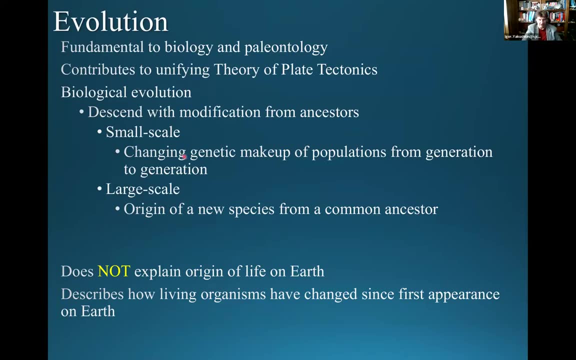 chloroplasts probably were uh free-living bacteria. mitochondria has been free-living bacteria which got been absorbed by the larger cell anyway. so now evolution again. evolution is the process, process of what? of changing genetics, genetic frequencies or genetic makeup of the population from generation to generation. 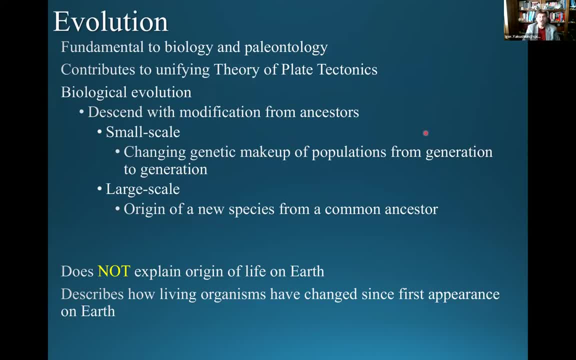 this is the definition i'm looking for when i'm asking about biological evolution, just saying change. change of what? change of genetic or process of changing the genetic makeup or genetic frequencies of the population from generation to generation. we already discussed that multiple times and this is what i'm looking for now again. you will see that exa, that that particular. 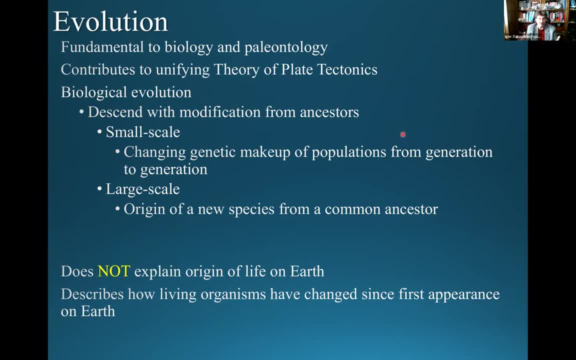 question: biological evolution pretty much every single time on the test lab, practical or the lecture test. now, in this particular case, what exactly? yeah, i i will be always looking for some sort of examples. i gave you several examples. i'll talk about several examples today as well. and again, theory of evolution has quite a large andек. 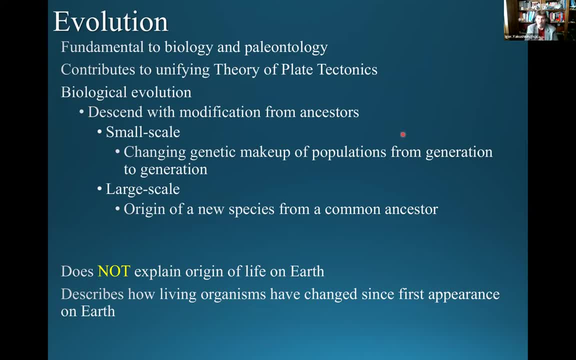 prz Allahu akbar. resolute theory of evolution has a broad spectrum according to dogms. amount of evidence. we discussed some of those evidence before and one of the problems is does not really explain origin of life on earth. we don't know how it started. we really don't. 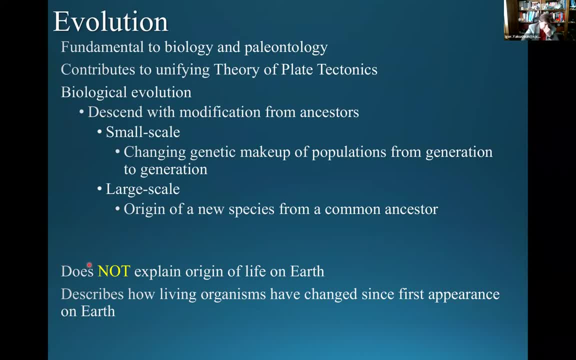 once again, some of the scientists saying the uh, the meteorite brought in, but it's basically how the bacteria got on the meteorite. some of the scientists saying that, uh, over a period of time, enough of the chemicals got together and they started that particular process of life. maybe, maybe not. well, there is a divine intervention, of course. um, a couple of. 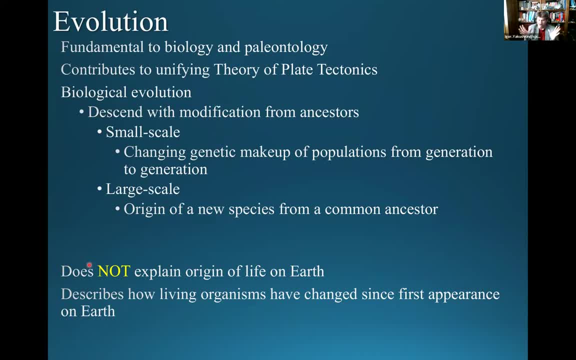 years ago i was traveling through california uh national parks, like you know, sequoia national park, and we were staying in yosemite and there was a quite a strange guy- uh, even to the california standards- next to us and we got talking and he was teaching at the local uh college as well. 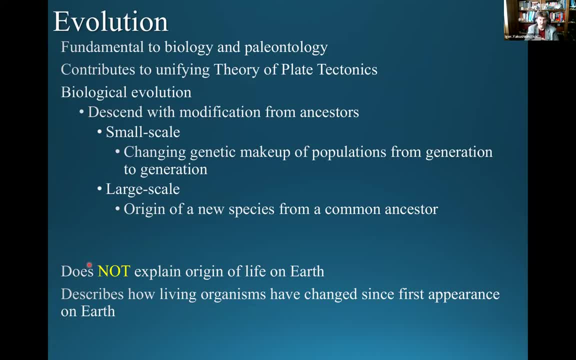 and he told, oh yeah, i know how the life started. i'm like how he like extraterrestrials were flying on the flying saucer. i'm like, yes, that's a good idea. yes, actually, and they decided to stop by the uh, stop by on that particular rock. you know kind of have a little picnic and then one. 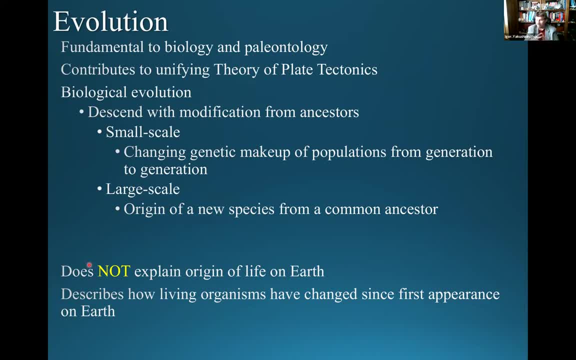 of them either vomited or spit into the ocean, and this is how the bacteria were, uh, were introduced to the um, new planet. i'm like, well, yeah, that's, that's interesting theory. not too much foundation, well, i mean with evidence of that. but yeah, maybe it happened. yes, and we are just 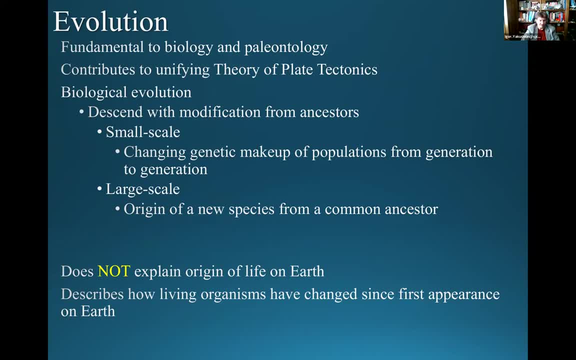 evolution of the extraterrestrial woman, or spit anyway. so what evolution does? it describes how the organism changed. remember changing in genetic makeup, small changes over period of time, and we'll talk about that, about the macroevolution. uh results in all kinds of different forms and shapes, creating the biodiversity we're observing nowadays. all right, so evolution? 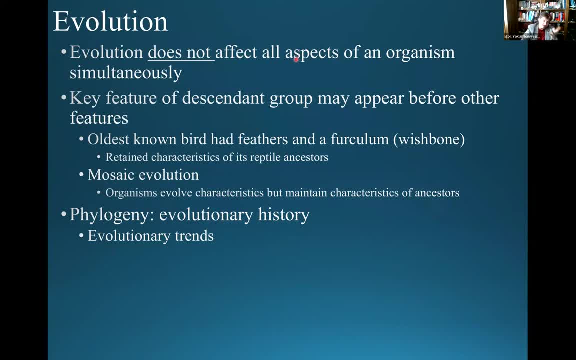 does not affect all of the aspects. on one hand, this is according to modern theory, or synthesized theory of evolution. however, we already talk about the back right. remember squeaky voice? uh well, high pitch voice, so to speak. if it's just uh, by itself, there is no advantage. 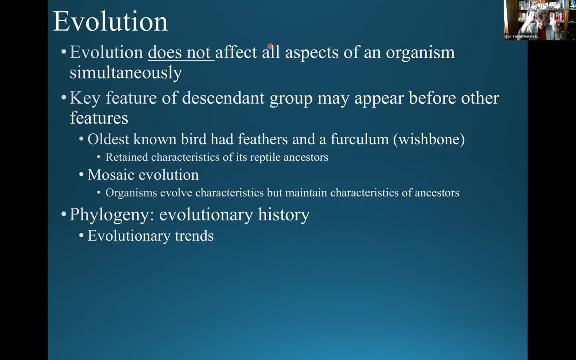 it have to develop a special years, have to develop a special part of the brain, and so on, so forth. so in this particular case, there is some of the issues. that's the reason why evolution is a theory, one of the things that are quite often nature. god, if you wish, uh, within evolution does. 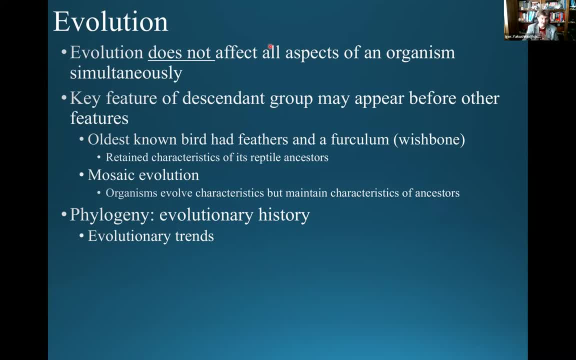 does repurpose some of the things like, for example: uh, before the, before the birds start flying, the ancestors, basically dinosaurs, already had a wishball and then it was a repurpose, so the muscles can get kind attached to that, the flying muscles, of course. now god and the evolution. 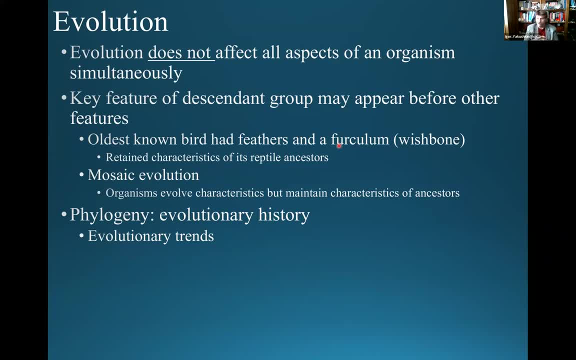 i specifically use that. uh, in the beginning of 2000, somewhere in that area, the roman, well, the head of catholic church, pope, come out and says: yes, evolution. well, i'm paraphrasing, but the general idea is: evolution does happen, the change within the living creatures it's, it's, it's been proven. 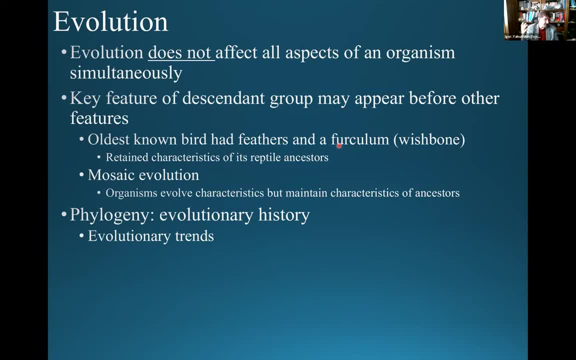 but it's all according to god's design and that's fine. he just provided the one of the possible mechanisms of the evolution. the problem once again: we can observe the evolution. why? it's a theory, because we don't know all of the mechanisms of the evolution. we cannot answer that. 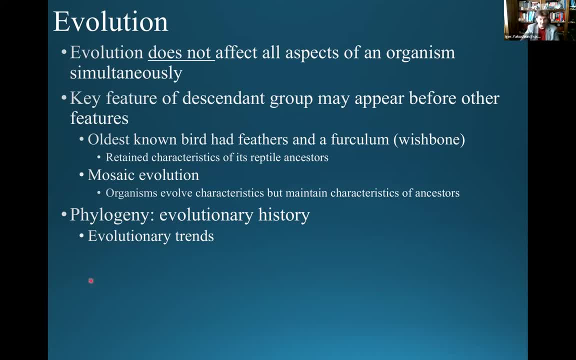 just yet. so, anyway, we'll talk about the phylogeny. phylogeny is: who is related to whom, and you did the cladogram assignment for that. and then, of course, uh, in that particular cladogram assignment you can observe some of the evolutionary trends like, well, four legs, that that's a trend for the. 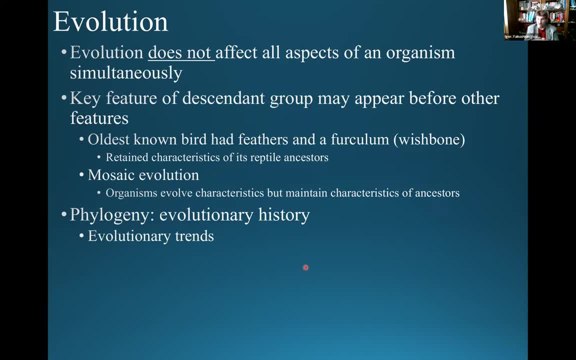 terrestrial creatures, all of them. all of us ended up with the four legs. amphibians started, we still have the four legs. you're grabbing the, let's say, a frog and counting how many toes it has. guess what? five now? uh, why? some of the organisms like, let's say, some of the dinosaurs, as well as the birds. 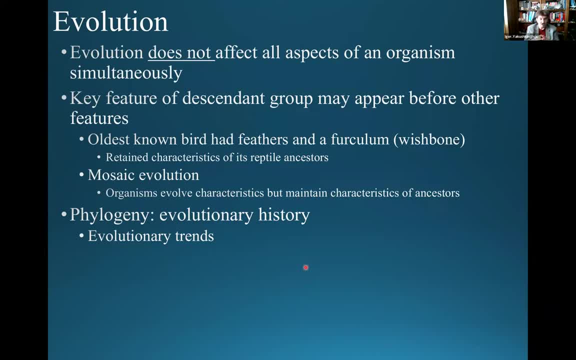 three, for example. well, once again, as long as it's not uh not disrupting the evolution, overall the number of the uh limbs will stay the same. but now think about it: our pink is already much smaller than, let's say, the um, the pointy fingers and so on, so they're slowly reducing in size and 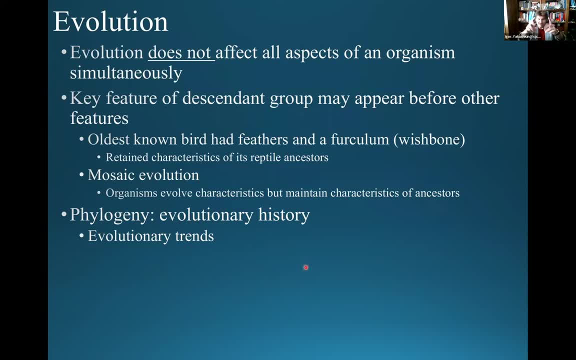 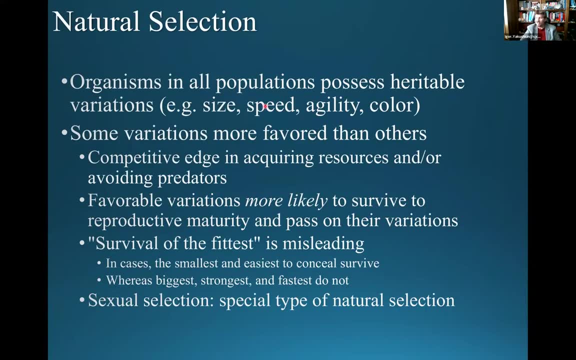 at some point of time we probably will end it up with three again, because you can text and do pretty much everything with only three, uh, three fingers, all right, so natural selection. remember that particular statement, survival of the fittest, is not entirely correct. surviving is important, but 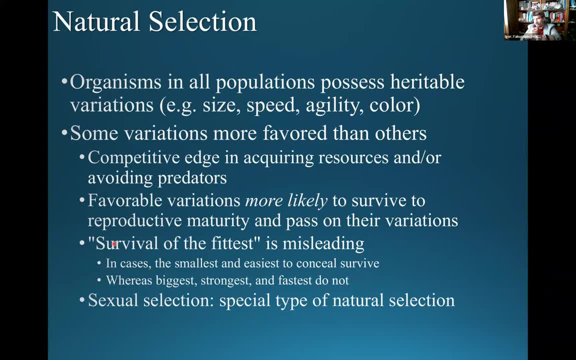 if you didn't reproduce. that's it, and this is where the biological species come. oh well, the definition of the biological species. come into your place. remember what biological species are: a population of the species that are in the place of the biological species that are in the place of the. 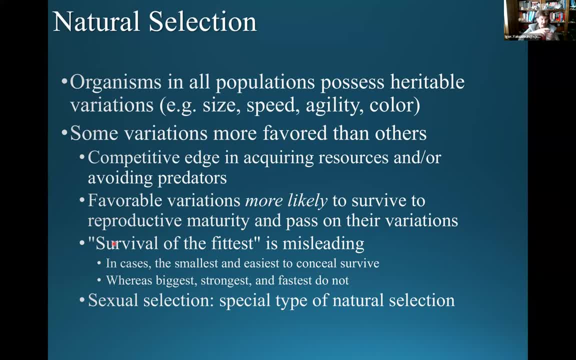 population of the organisms capable of interbreeding. interbreeding is one very important step, but also a produced fertile offspring. some of you, when you are writing that particular answer down- biological species, uh, capable of interbreeding, and you stop. no, don't stop. continue produce. 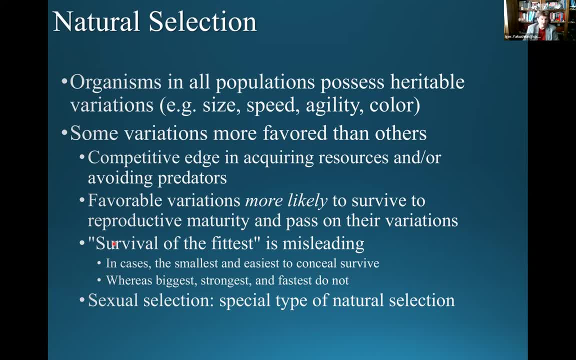 fertile offspring very, very important, because if it's an infertile offspring, the next generation, all of those uh fitted things would be gone, literally destroyed. they will die off with the carrier, so to speak. so be very careful on that. and once again, the biological species, that particular, with the examples, plural right make. 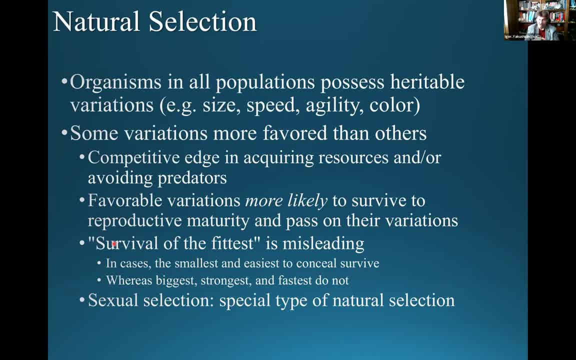 sure that you will be able to uh provide some of the examples: wolves, coyotes- we are coyote right in the college. that's the mascot. and then there is the ravens, and then there is alligators. i think it's a north one. anybody knows what's the uh mascot of the new one, the generation park- anybody? i? 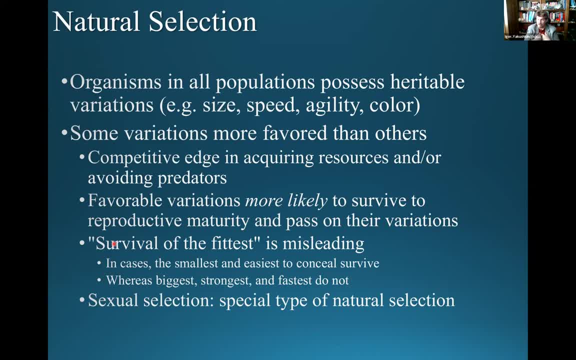 have no idea. i honestly don't. so survival of the fittest: even though darwin proposed it, it's slightly misleading. sometimes smallest is easier to conceal and survive. sometimes the biggest one will not be able to reproduce. they're a for not only survival but also the reproduction and then, of course, sexual selection we talked about. 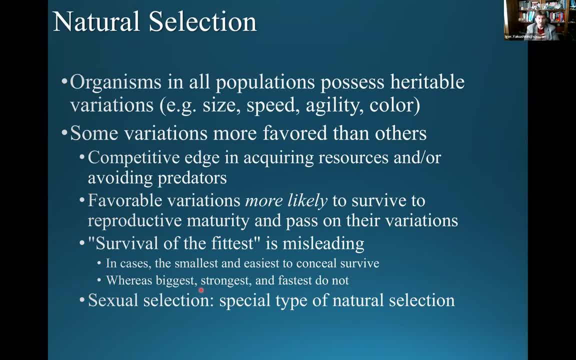 the hardy weinberg equilibrium. remember all of those particular five major traits in order or conditions for the equilibrium to be. it most likely will be on the lab, practical, so refresh your memory on that. and yeah, there is not real world population which is in equilibrium, none. whatsoever. it's. a third of us are supposed to be in balance between life and death, but we have a number of species, so in the first place, there is only one life, and when we die, there will be no survival, and this is because there are two of these species. this is the last one and the second the first one. 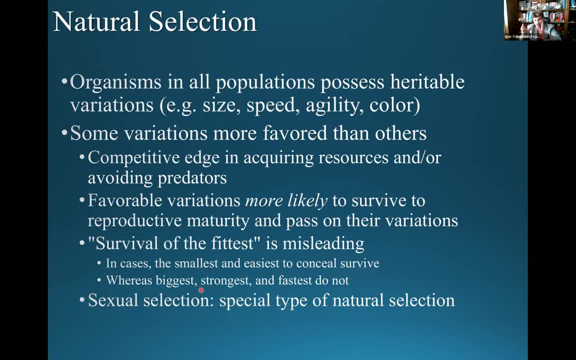 theoretical model, for us to use it against the actual data in the field, so to speak, so we can say, yes, the uh generate. well, the genetic frequency is changing. yes, evolution taking place. so, yes, sexual selection is a special type of natural selection. by that we're talking about random. 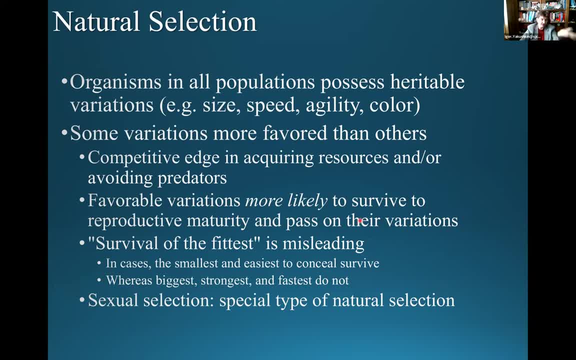 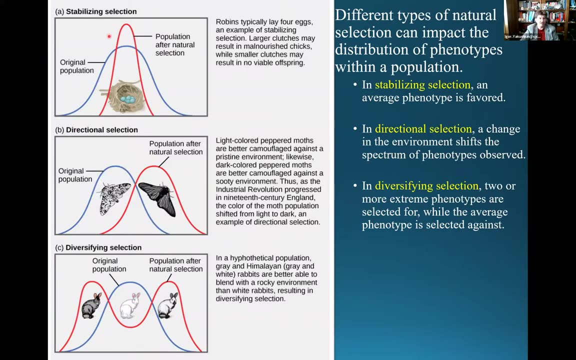 versus non-random mating. for the equilibrium to be, it have to be a random mating. sexual selection means that there will be a preferences, all right. so several types of natural selection. one of them is a stabilizing natural selection. stabilizing natural selection are favoriting the medium. 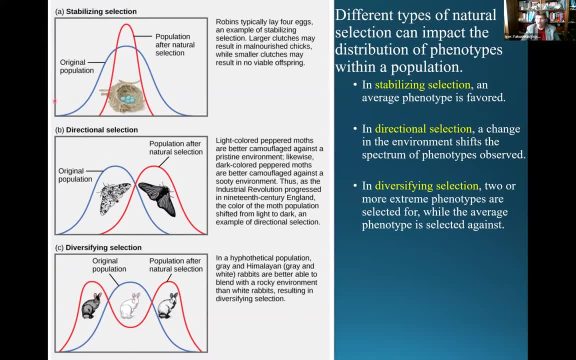 the average, that's basically average- phenotype is favored and in this particular picture it shows you the number of eggs in the clutch. so if it's only one uh egg, then there will be not enough offsprings, uh, to carry on. if there is like 10 of eggs in the clutch, there will be well some of them will die. 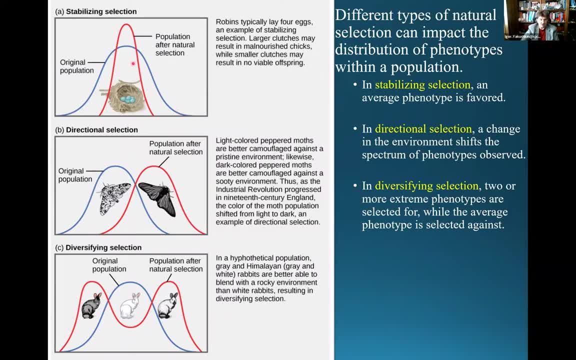 off from not being properly heated, so the average is good. now directional selection, and we'll talk about that and that's a really it's kind of iconic example of the evolution and it's also example of the process of evolution. so what exactly we have? this is the original population. 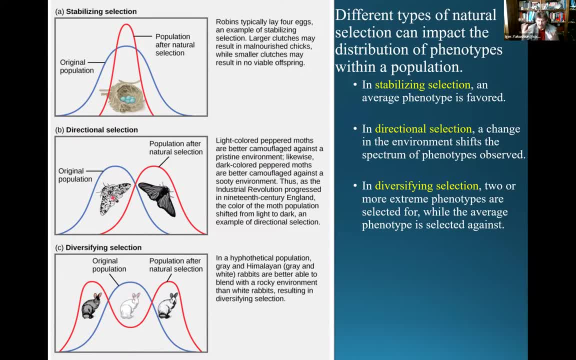 peppered moth. peppered moth is the butterfly kind of type of the creature which, uh active during the night, during the day it sits literally sitting down on the bark of the trees and because of its speckled pattern it's kind of hard for the predators to see. 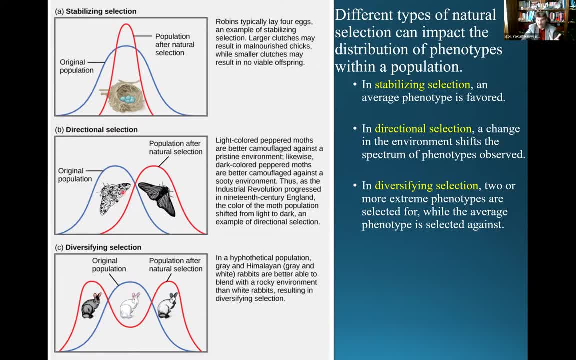 in the late 1800s in some of the areas of great britain scientists noticed that they start seeing much more darker variety than the original one. and they said why in the world we start seeing the darker versions not everywhere, in the particular spots? so they start, uh, figuring. 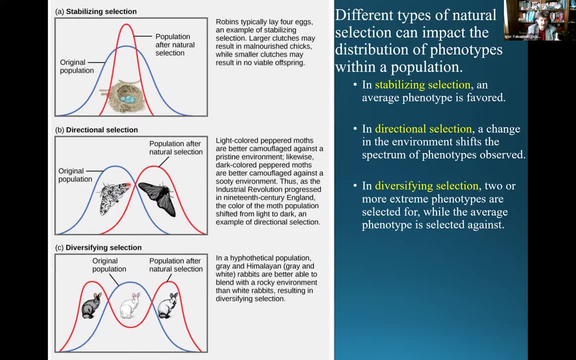 it out and what they uh ended up with? that in the areas which are heavily- uh heavily- polluted by the suit, industrial revolution right burning coal to produce energy. whenever you're burning coal, the suit comes out and then it settles down in the environment, including the bark of the trees. 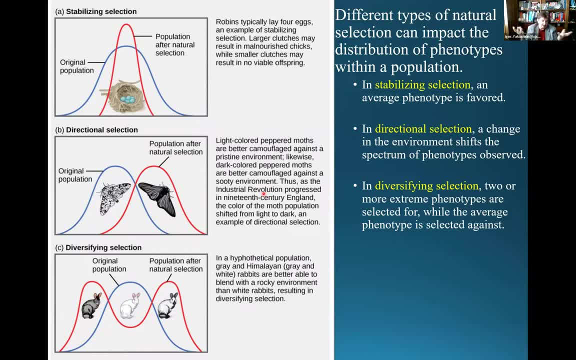 now, over a couple of decades, we start seeing the tree bark. the color changed drastically because of all of that particular suit. it's become darker. so the darker variety has the um has the ability to conceal itself. better it conceals itself, better it will be able to. 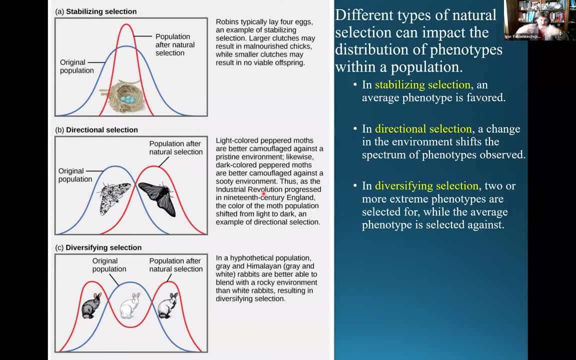 reproduce, produce viable offspring. and here we go. the next generation will start seeing the darker variety prevailing, so to speak, and further on. and then there is a diversifying selection. diversifying selection, it's kind of opposite of stabilizing selection. stabilizing goes for the means, the averages, when the average of the number of birds that will then increase the diversity of. 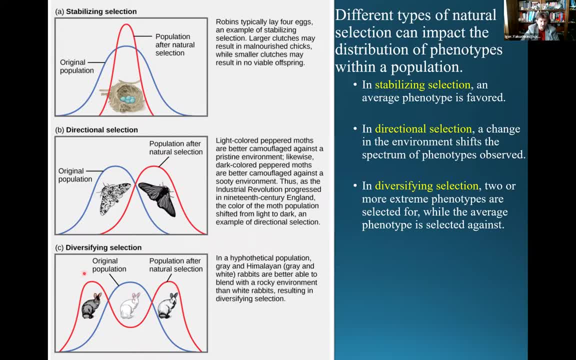 the stabilizing goes for the uh. the other ends the. in this particular case we have the original population and then we have the speckled, the bunny and then the darker bun. so those ones would have the lower probability of not only survive but producing those springs and that one will have. 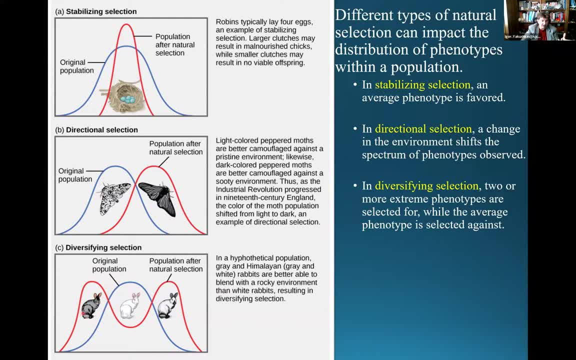 a higher, why, where rocky environment, you can see on the rocks all the the predator will see on the rocks they divide bunny very, very easily, right? so rabbits, uh, the gray ones will be, uh will be blending in better. on that one, for example, it's a snow fields where you have rocks and the snow. 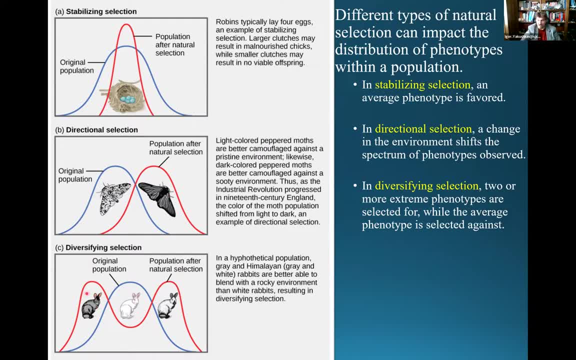 that one will be able to conceal itself better as a result. we're looking at the favoriting selection is favoriting the outsides, and then, of course, those particular bunnies over a period of time, and those bunnies will separate, there will be a geographical barrier between them and then 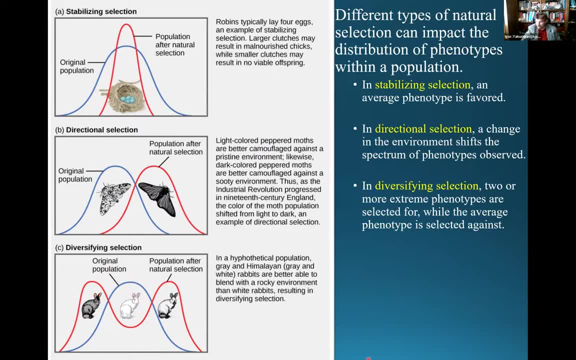 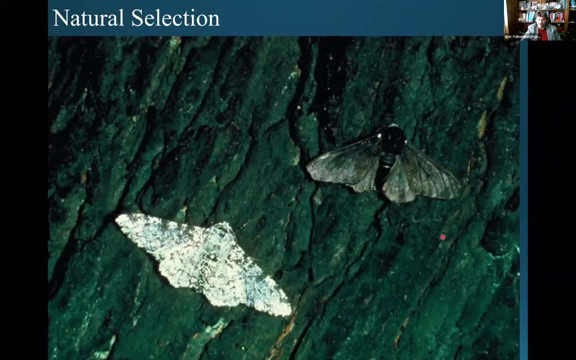 eventually will become close related species. the next picture: here we go. we're looking at the normal peppered moth and the darker variety on the suited bark of the tree. so in this particular case, if i'm looking at the dark area, i will see that one much easier from afar than this guy. there are four that 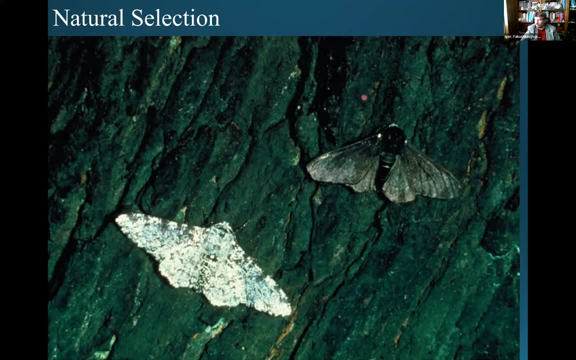 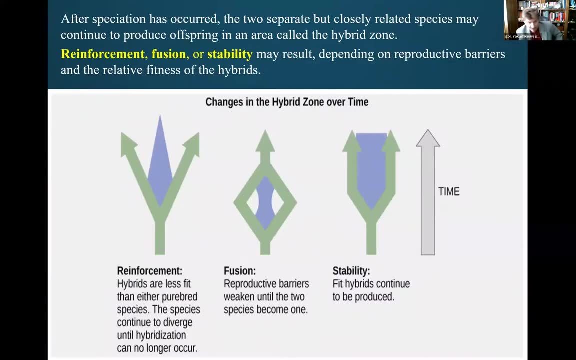 one will be eaten, that one will conceal itself, will be able to reproduce, producing more darker varieties, right? so here we go. that's example of what of the evolution: peppered moth, uh, darker variety. so here we have several major, uh major trends in the hybrid zones. remember the population. 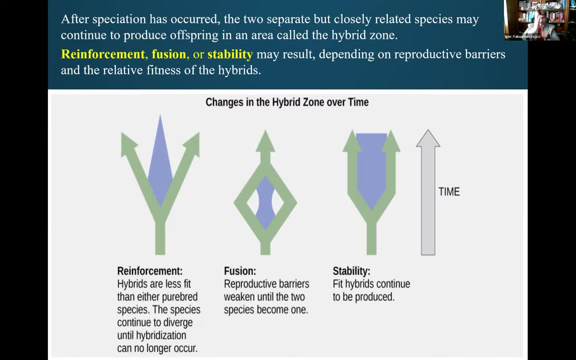 splitting apart. so the population is split into two different species and we have the same species, but they are splitting. there might be some sort of geographical, uh- barrier between them, maybe some behavioral or anything like that. three possibilities: first of all, the populations are splitting and then over a period of time, the hybrids are created by over a period of times. 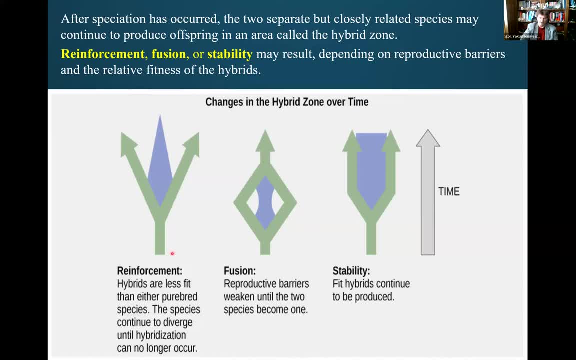 less and less hybrids will be created. therefore, eventually we'll end up with two new species. it's reinforcing the natural selection and essentially the process of evolution, now a speciation, a process of formation of the new species, now fusion. we start with two- uh two- populations, and then they. 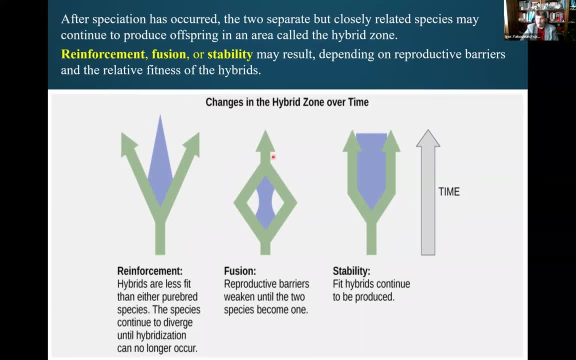 merge back for one or another reason. so now speciation basically stop. they start exchanging the genes very nicely, and here we go, we continue to have one species, and then the next species is the new species, and then the next species is the new species. so we have uh. 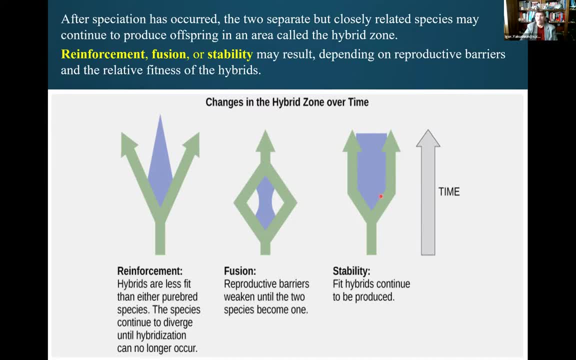 population number one, population number two, going into a species number one, species number two, each one of those producing the hybrids. hybrids continue to produce, but quite often hybrids will start, uh, start interacting within the hybrids, so to speak, and therefore you might end it up eventually with the third species, which will be related to both of those newly species and of. 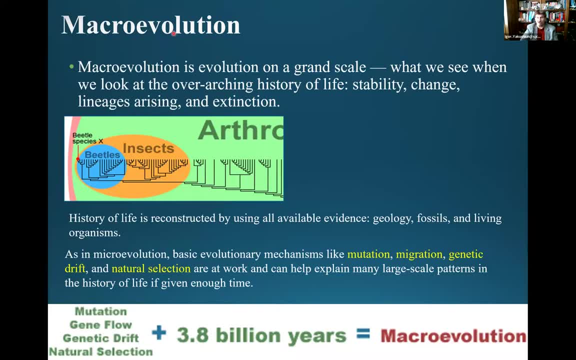 course, the last species. so we have the这个. the sql often is called the ongoing evolution and it fundamentally requests a large-scale, small scale change in the shifts in the evolution of the populations or in the population and so on. we looked at the evolution of populations and some of the 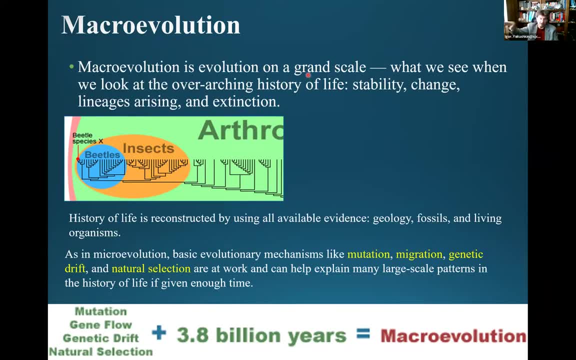 collaboration between the species. this causes the mass evolution, the population and so on and so forth. so that's the requirement. so here we go, the macro evolution, a large scale, starting with again micro evolution, talking about the genetic uh changes in the genetic frequencies within a population, everything above the population, species. genus, etc. that would be a macro evolution. so essentially, remember mutations. essentially we're taking those particular equilibrium conditions, saying no to the mutations we're not going to. that's the specific content i'm going to show you. next slide. so that's the specific content i'm going to show you. that's the specific content. 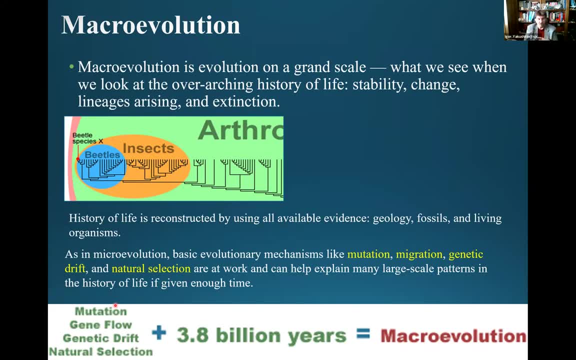 no mutations, no gene flow, no gene flow, no natural selection. now we have a natural selection, all of those conditions, plus quite a large amount of time- 4.2 to 3.8 billions of years- and now we're looking at the evolution on the grand scale: macroevolution. 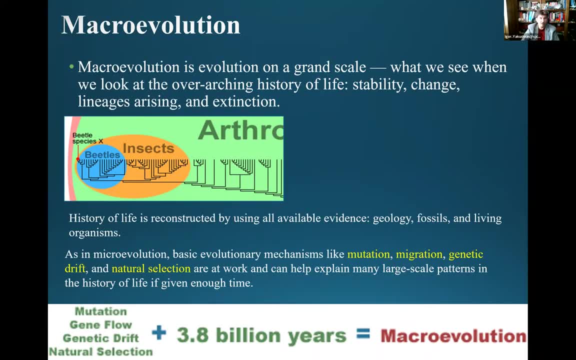 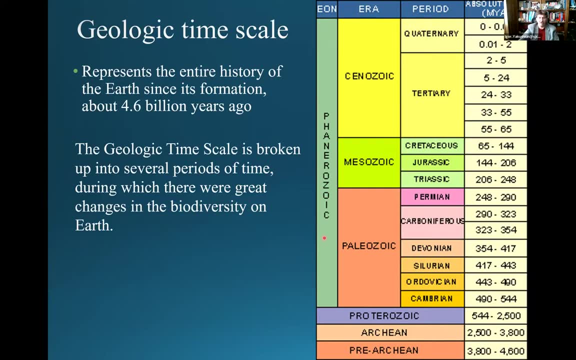 all right. so geological scale: this is kind of a little bit of geology. my background is also in geology. i have a zoology and geology background. i have master's in geology. used to teach geology at the saint jack, but if we look, you don't have to memorize. i'll show you several major things. 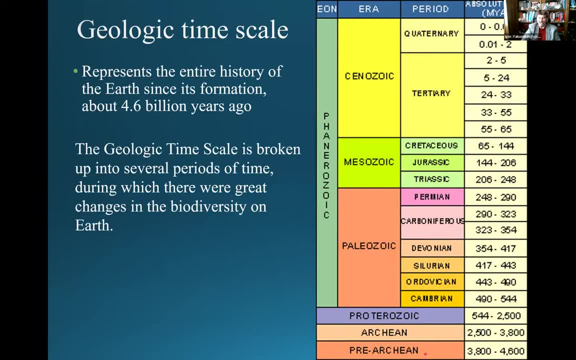 uh in here, but pre-archaean. archaean means ancient one, archaic, pre-archaean, that's basically before the life started, essentially arcane and proteozoic. we start seeing the life, some of the signs of the life, but mostly it was either uh, a bacterial one. 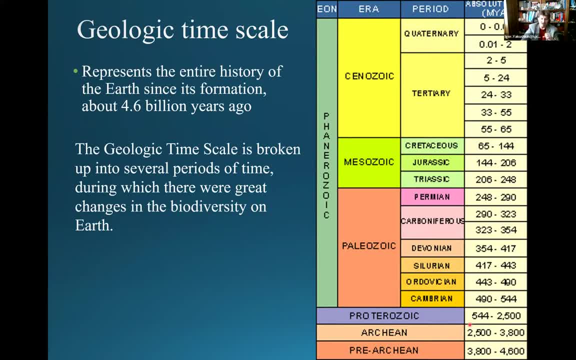 so prokaryotic. somewhere around here, most likely we start seeing eukaryotic cells. but everything was on a single cell level, so not much of the fossils remain. soft tissues generally do not preserve too well. all right now here look at this particular period known as the cambrian period: roughly 550 millions of years. 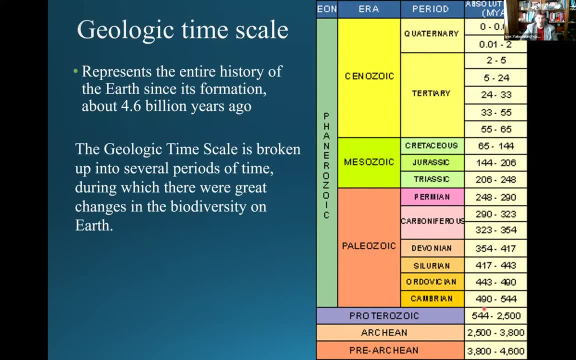 ago, we start seeing something which known as a cambrian explosion- explosion of life, different shapes, different forms. as a matter of fact, out of 40 plus phylum of modern organisms, about 90, 80 percent- excuse me, 80- can be traced back to the cambria. 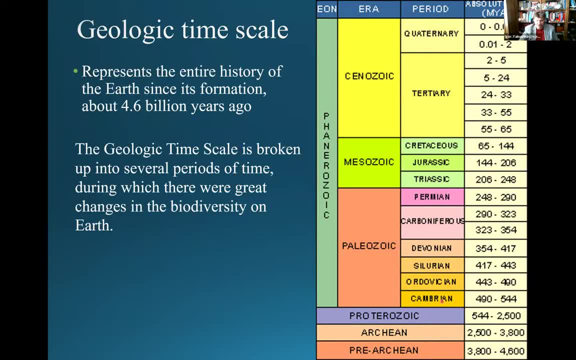 and that's known as a paleozoic ancient life, everything going right. here we'll talk about the carboniferous era. this is where we start seeing the um, the increase of the land, plants that they started somewhere in silurian, maybe our division and then, but they uh. 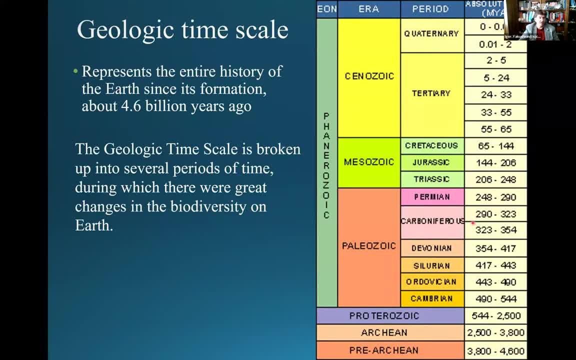 gradually went up with many generations, such that, as we move forward, the puedo perceptions of Что так? there was a super volcano, most likely a super volcano was erupting. it was. a fissure volcano means a crack in the land for about thousand miles long, and it was. 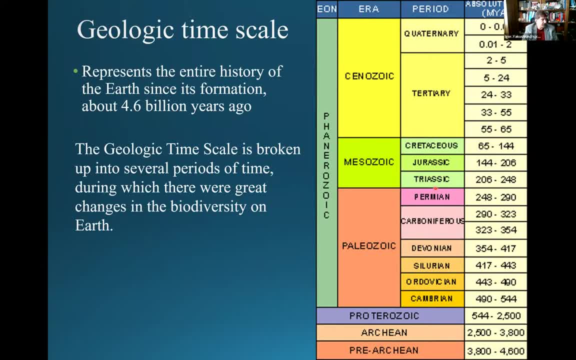 oh well, it was erupting for about a million or so years, filling up the the atmosphere with the toxic gases. as a result, about like 90 percent of the marine life died off, or we were very close to, well the life were very close- to be killed during that particular time. 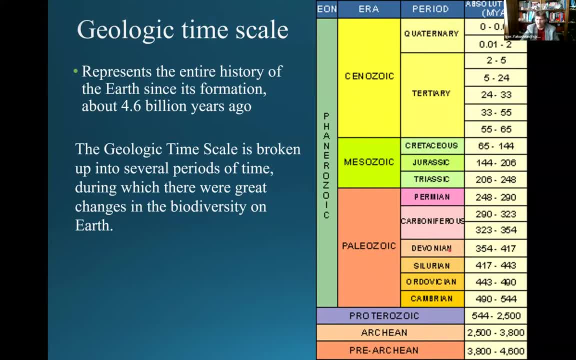 and then, well, there was a few other. we'll talk about a few other extinctions, but permian was one of the largest ones. and then, after the permian, we start seeing the race of the dinosaurs. everything was good until the 65 millions of years ago where something happened. we had another mass extinction. 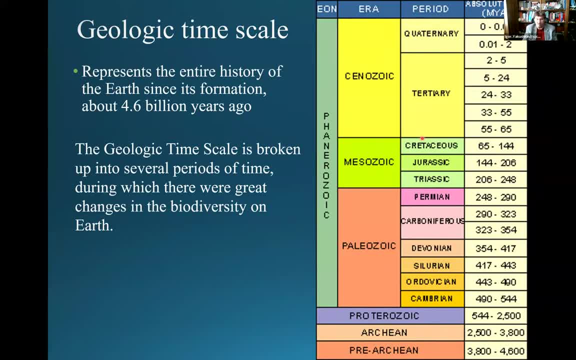 and most likely it was the meteorite. meteorite plus super volcanoes, uh any combination of that, and then we start seeing the rare arrays of the mammals. so we'll talk a little bit about that. that's quite interesting how geological uh events shaping the uh diversity of life. so here is the 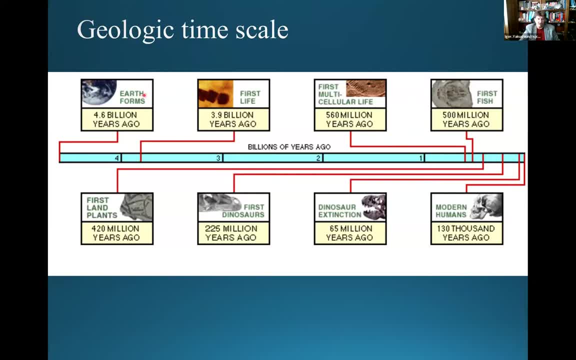 geological scale, but it doesn't just explain the numbers we just learned about. the earth competes in 6 billion years, so that's the native resides of the professor george cuneo. good evening, i'm ben richard from the german학j forskj Sesame �umi. 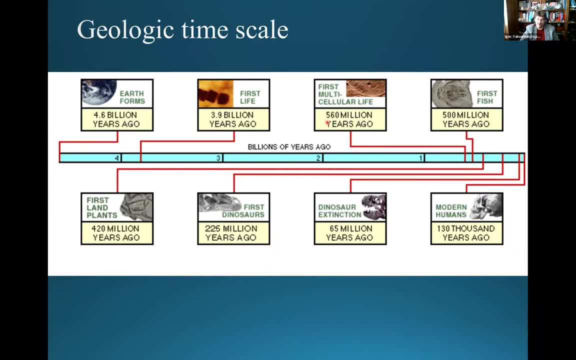 and we are in this one was one of these databases- to� billions of years, uh, within evolution, and then of course, we start seeing, uh first fish, and then first land plants and then, of course, the first dinosaurs, uh, the first mammals arrived on this particular, evolved on this particular earth, around 215- 200 millions of years ago, so they kind of were. 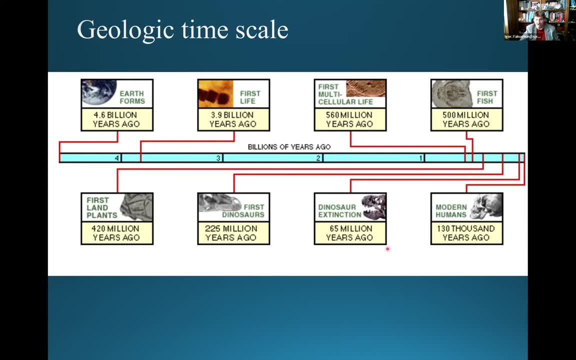 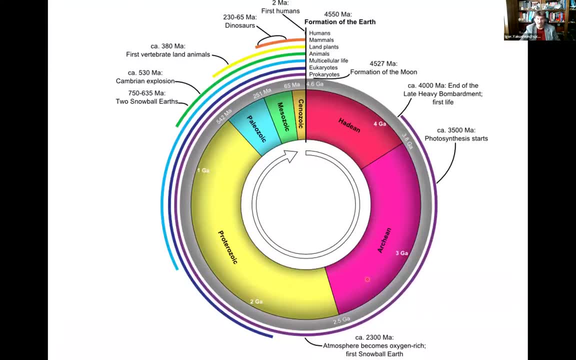 evolving in the shadow of the dinosaurs, then the extinction of the dinosaurs with the following proliferation of the mammals. now you already seen that particular picture kind of gives you all of those ones in a nice circular, uh kind of pie graph, uh scale. so a law of superpositioning. 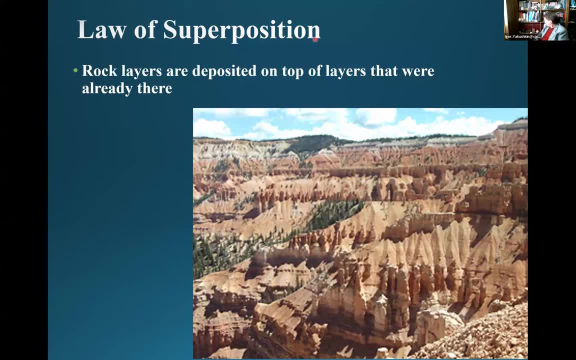 if you're ever interested in any kind of works, and you can say i have several of them on the background. once again, i was teaching geology. a law of superpositioning is one of the crucial laws. now, it's a law, it's not a theory in geology. 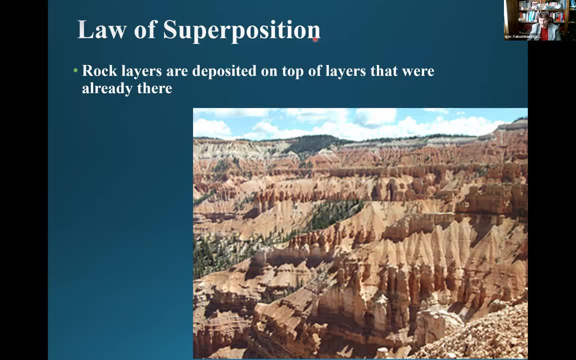 and this is one of my favorite, one of the favorite national parks in the united states called the zion. oh no, it's not that it's right next to the zion national park, but three hours uh up north. that one is a bryce canyon, a really, really beautiful place, and you can see the law. 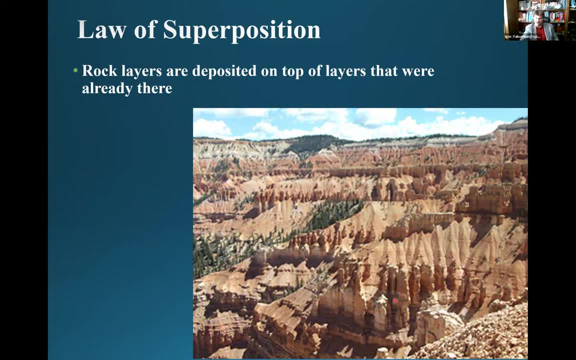 of superpositioning here. very nice, you can see the layers, different layers, on that particular canyon, and the deeper the layer, the older it is. that's all. the of law of superpositioning says that in the ocean, whatever settles on the bottom, whatever is on top, is younger than whatever is on the bottom. that's. 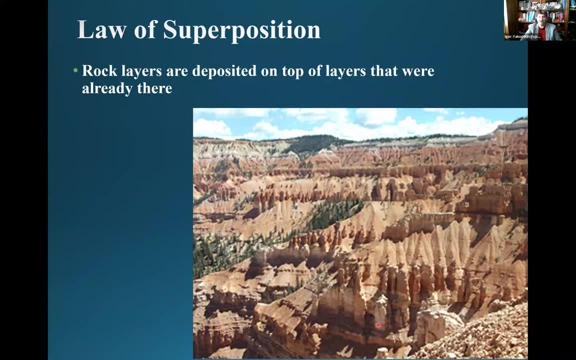 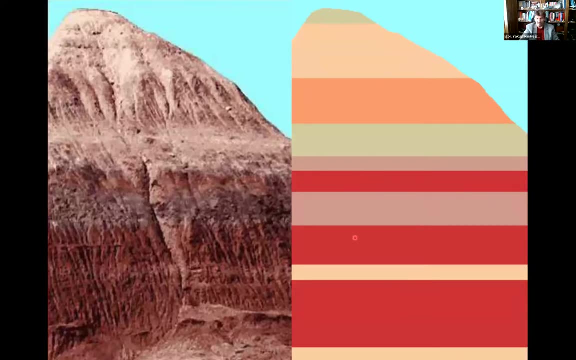 pretty much it. so rock layers deposit on top of the layers were already there, meaning they are older. how it's applied to the uh, to the biology. see that one is the oldest one, this is the youngest one and you can say that that particular layer is uh, that layer is younger or more recent than this particular layer. but this layer 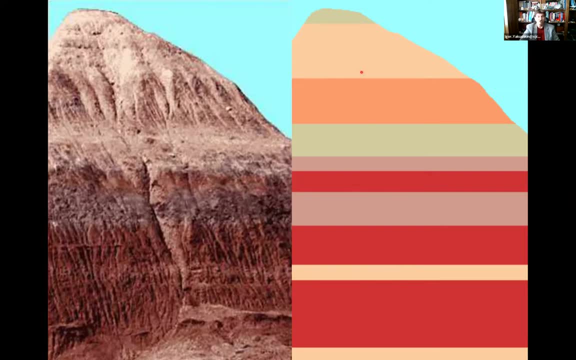 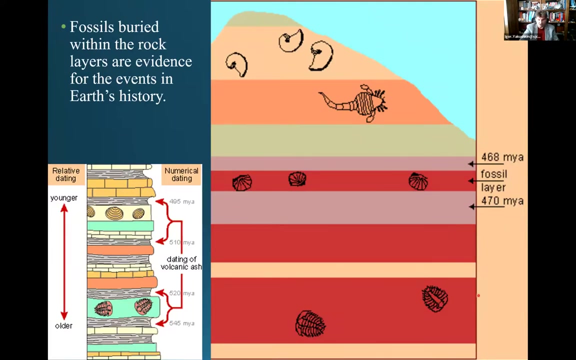 is more recent than that one. so we can do some sort of relative dating. we can say: this is the youngest one, this is the medium one, this is the oldest one. so now, if we'll use the creatures in there, we'll look for the fossils. we can say that those guys, the trilobites, are older than those. 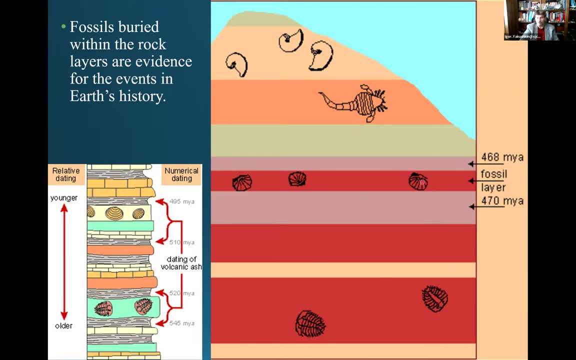 guys they are. they're older than those guys. they're younger than those guys. the older ones are something which is known as a brachiopod, but brachiopods are older than the eurypterids sea scorpions and the sea scorpions are older than the nautilus. can that make sense also there? 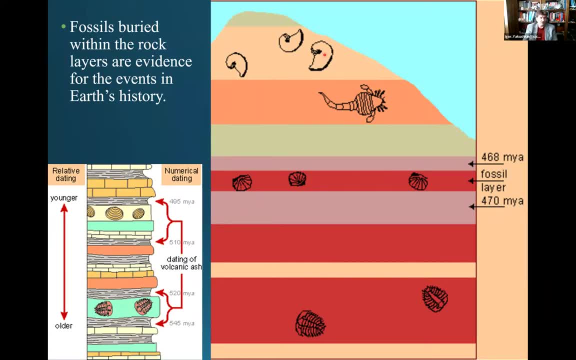 is another uh law in. well, it's not. the law is a rule of thumb in geology that we generally cannot date the accurately sedimentary rocks. there is a several types of the rocks. there is a hard rock, no, no, there is a igneous rocks, sedimentary rocks and metamorphic rocks. so, uh, we cannot. 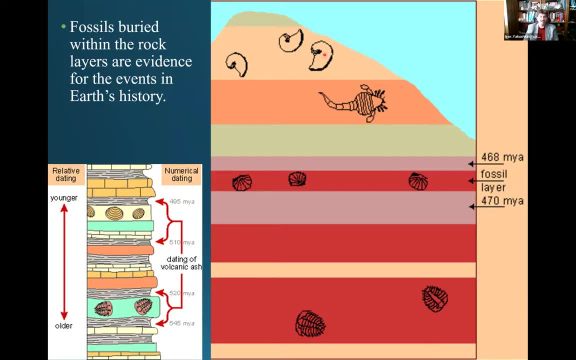 date metamorphic rocks accurately and we cannot date the sedimentary rocks accurately, but we can do the um the igneous rocks relatively easily using the different radiometric date. so in this particular case, one of the types of igneous rocks, like volcanic ash or volcanic flow, like lava flows, those ones we can date pretty accurately. 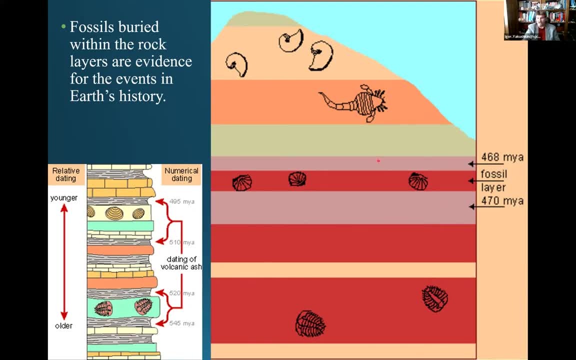 as a result, we can say: well, this is a lava flow or volcanic ash which is 468 millions of years, so everything above that will be younger than 468 millions of years. everything which is below will be older. now look here. we had two layers of igneous rocks. one of them is dating 468, another 470, and the layer in 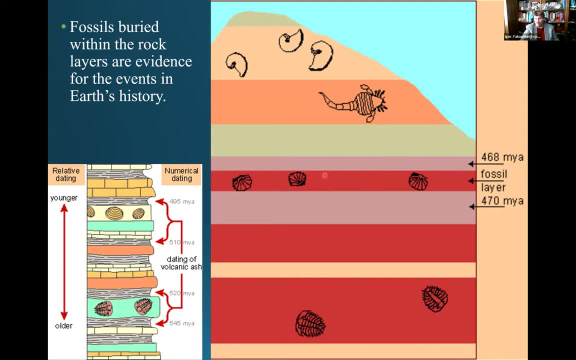 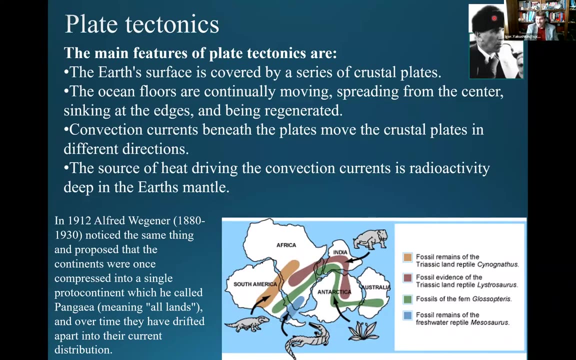 between. we can say pretty close that those guys somewhere between 468 to 470 millions of years old easily, uh easy, right, so late tectonics that particular gentleman, alfred wegener, come up with crazy at his time, an idea he actually in 1912. 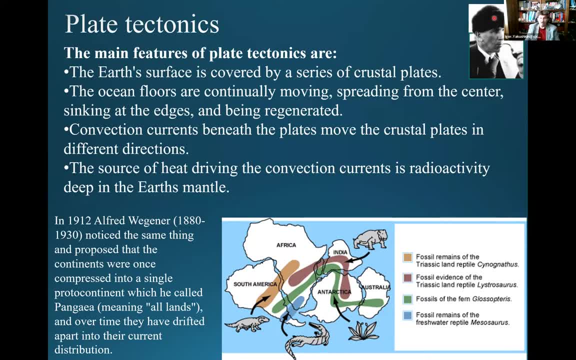 he published a paper. he said, guys, continents are moving. and everybody's like: what are you smoking, man? uh, and he's like: no, no, no, i'm telling you that africa, south america, antarctica, australia, as well as india, at some point of time where a huge continent, he actually called it pangaeano- 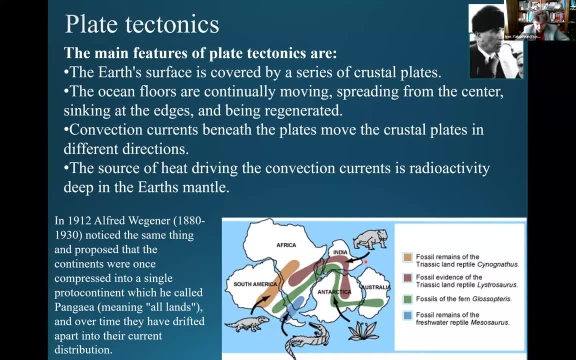 means all. ga means earth. all earth was a one huge super continent and then it broke down and they like how in the world the continent is called? so i mean, is that it's, it's and some moving and feel like i don't know? i just kind of noticed that the uh, it's actually well. 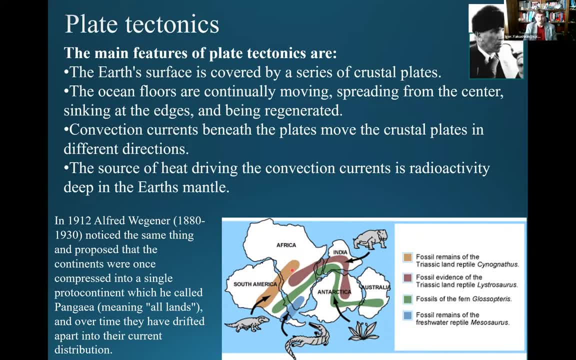 first of all, the outlines of the continents, now tectonic plates, are matching and second of all, we can match the specific fossils, like, for example, there is a particular fossil of kinda relatively large land reptile. think about huge lizard. it's not a lizard, but uh, you can find it in africa, in 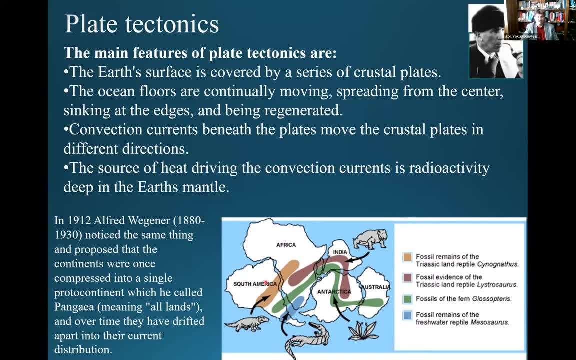 specific areas in africa, kind of central africa as well as the central of south america, not central america but central part of south america- and there was no at the same levels, at the same uh type of the rocks and there was no explanation how in the world the same species of the same uh. 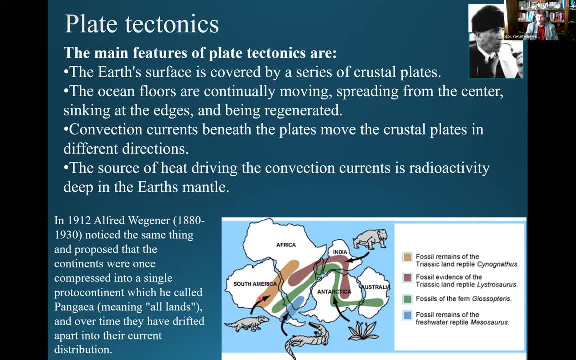 reptile were able to move between two huge continents, until that particular gentleman says: well, at some point of time they were connected and therefore the reptiles didn't have to swim through the atlantic ocean. it just it was a single continent. same thing. we're looking at the another land reptile and that one, something which 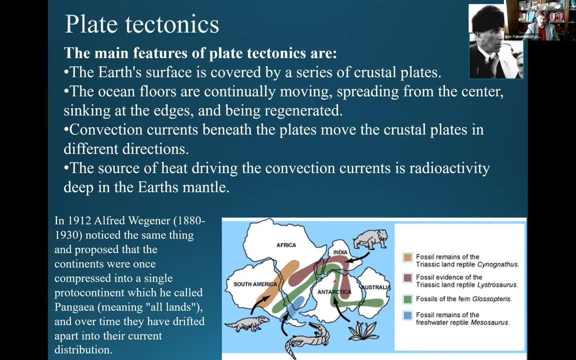 known as the glossopteris, will see that particular the uh that's. that's known as the fern tongue fern and that's where the reptile one is coming out. the other is the has a common tonged turd. that's the particular tongue fern uh fossils you will see during one of our labs later on in both so he 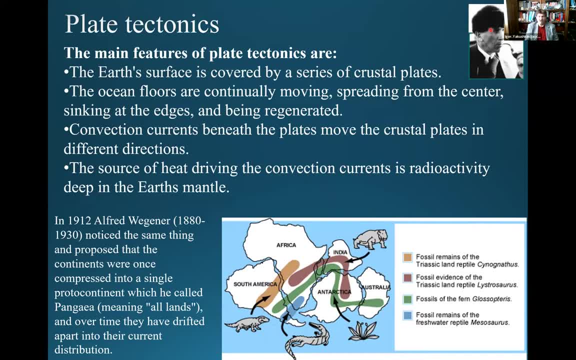 could not explain. now we still kind of it's a theory, we think that the uh plates are kind of floating on top of the mantle or on top of the magma and they're slowly moving. now we do have the evidence that the plates are moving, but they are moving very, very slow, like for example, 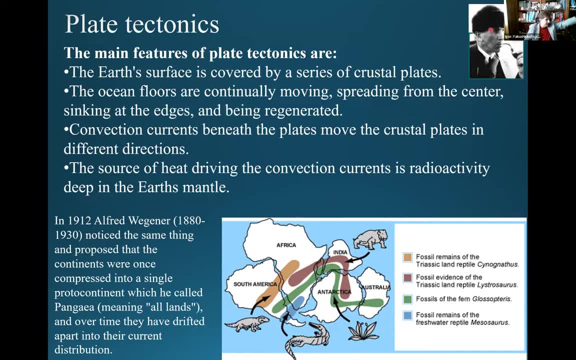 right now, north american plate, uh, with a whooping uh speed of one inch a year, goes toward the asia and eventually they will collapse, yay. so if you are decide it will take couple of millions, but if you'll decide couple of millions from now, uh, decide to, let's say, invest in. 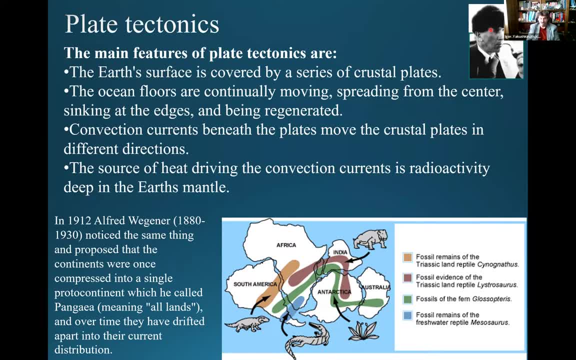 japanese real estate market. it's not really a good idea. why not? because of japan, islands of japan is right in between two continents which will be colliding and of course there will be like volcanoes coming out, the godzilla will come out, all that particular stuff, total destruction, all this uh thing. well, and this. 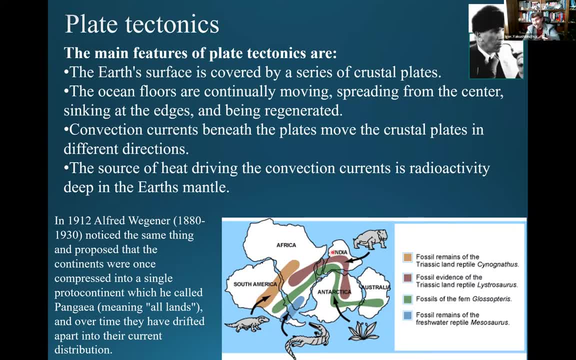 is what happens actually with india. india not as a country, but the continental plate. it starts moving and then eventually it collapsed or it's collided with the asian continental plate and they start raising up. now we have the highest mountings in the entire world, known as the 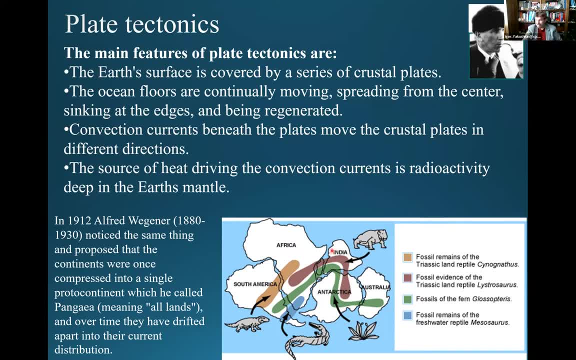 himalayas because of the collision of two of those plates, and that's explained why, for example, if you're going 8 000 meters above the sea level, you know one of the highest or one of the highest mountings in the world. you will be able to find. 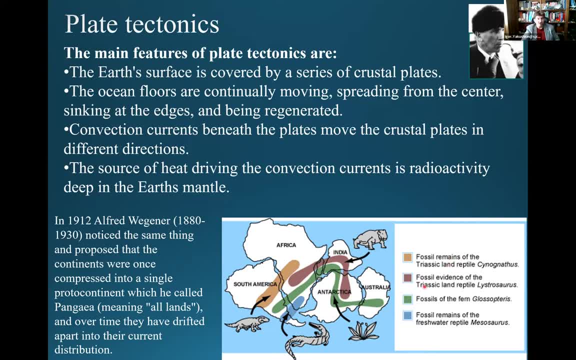 you literally a sea, uh, sea creature fossils on top of the everest, well, under the snow, under the ice, if you look, if you'll get into the uh, into the uh rocks, you will see some of the. some of the rocks might contain a sea creatures. how in the world, on the top of the world, we ended up with? 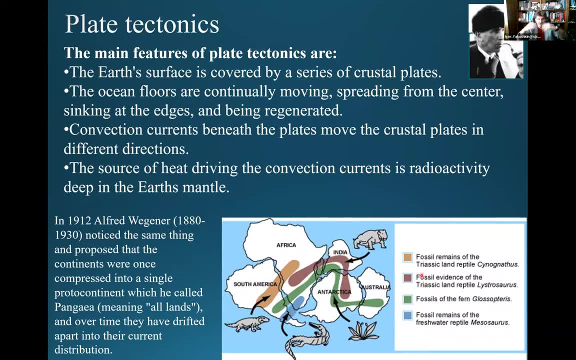 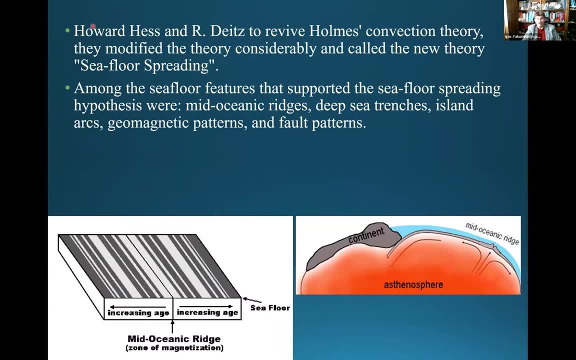 the sea creatures. well, because it brought it up during the collision, some of the sediments has been raised up by the collision anyway. yes, and the hovard has, as well as the dates, come up with that particular idea. we have the mantle athena sphere. athena sphere is moving slowly and this is what creates the movement of the 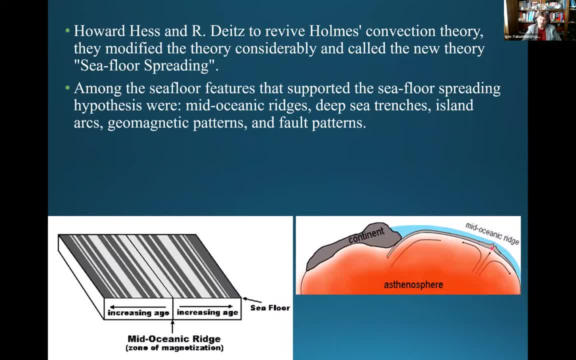 continent. as a matter of fact, athena sphere, mid-oceanic ridge, creating the oceanic plate, and we're talking about much more in the geology about that. so if you're interested, we are still offering his physical geology, which i like, but uh, i'm not sure if you're interested in. 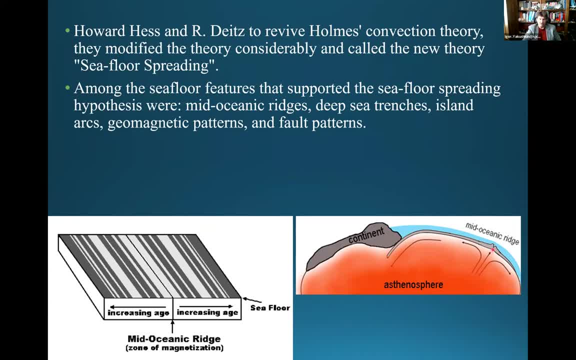 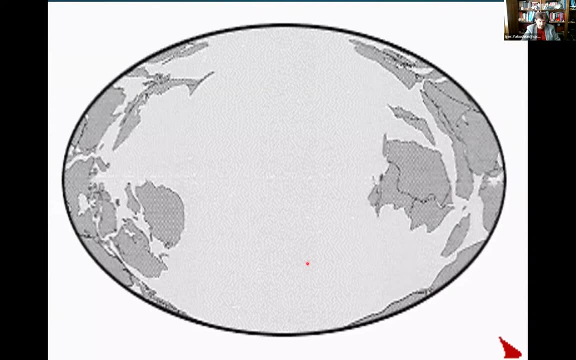 that i was, uh, much, much more interested in the historical geology. after all, it's my background. historical geology was quite a fun class. i'm not sure if they're still offering it at the well every semester at the south park, so let's kind of take a look. uh, we have. i need to remember how to. 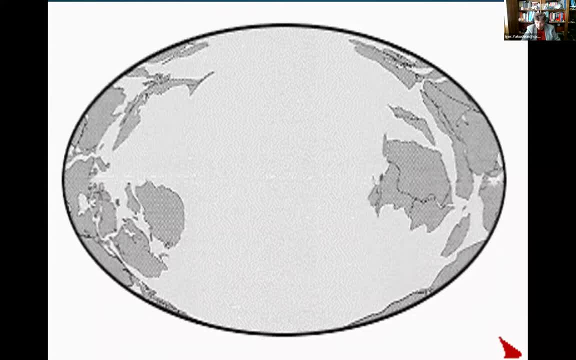 uh, i think this our controls. oh, here we go. so what you will be looking at is like 500 millions of years of movement of the continents in less than like 15 seconds. so let's kind of see how the continents, those particular pesky ones, were moving in the last hold on. let me get the part of 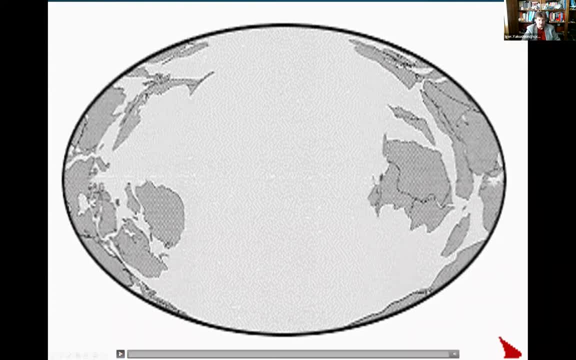 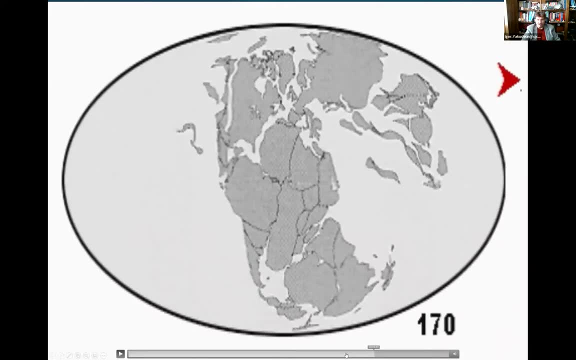 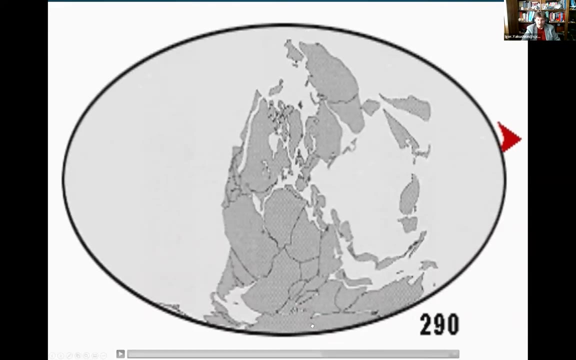 there we go, so let's kind of slowly say pangea and then it splits up very interesting part somewhere right here. you can see that about 300 or so millions of years ago we had a very huge continent with a very large, very large uh seaside or uh oceanside, so it was wet and warm environment. 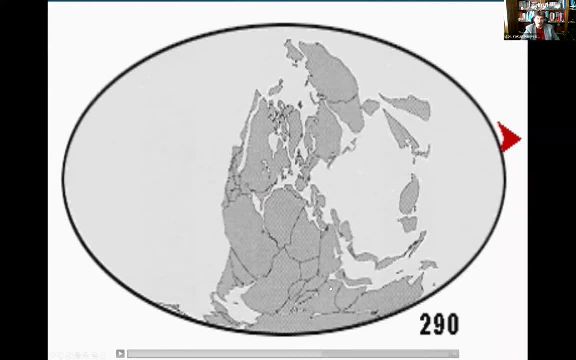 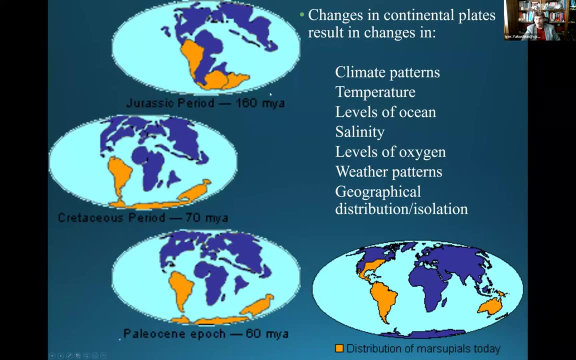 during that particular time which will give a rise race of uh for the plants, and we'll talk about the something which known as the carboniferous period. so here we have a jurassic park. it just kind of jurassic period. you probably heard jurassic park again. we have kind of single 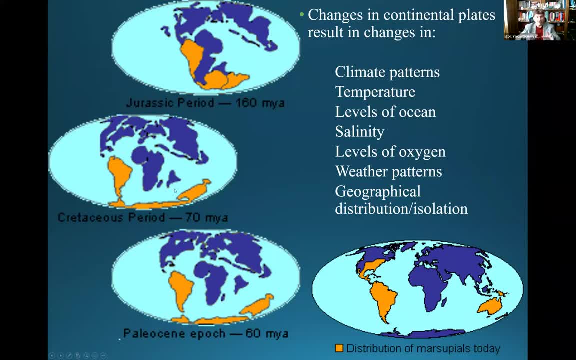 continent which start breaking down slowly because of that particular movement, and again continuous, even until now, the horn of africa is actually moving away from the africa. that's why we have a rift valley right there and few millions of years it will be filled up with the ocean. 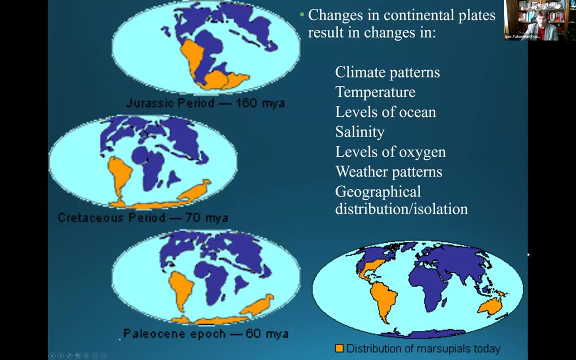 well with this inner well, with this salt water on the central ocean, and so on, so forth. now marsupials, let's say the orange distribution of the marsupials. at some point of time they were quite nicely populating the area of south, modern south america, antarctica, and then, of course, 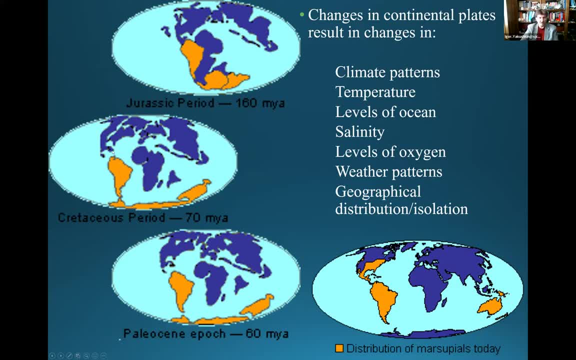 australian oceania. whenever it splits, it stays- uh. the marsupial stays on the north south america. well, they start dying off here because of the uh cold conditions and they stayed in australia later on whenever we ended up with the bridge between the north america and south america. we'll see that. 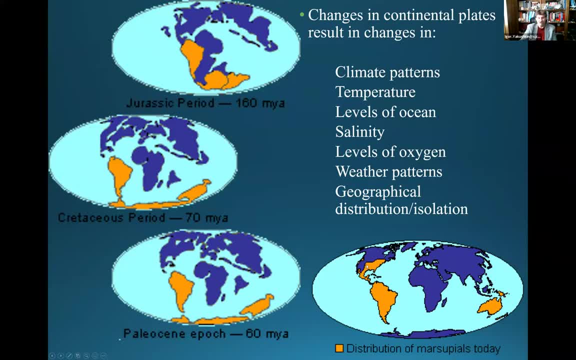 some of the marsupials actually moved in into the north america. most of the marsupials has been eliminated by the placental mammals in both of the americas. which marsupial we're talking about? a post opossums are the only marsupials- which is fine, as far as i know- which can be found. 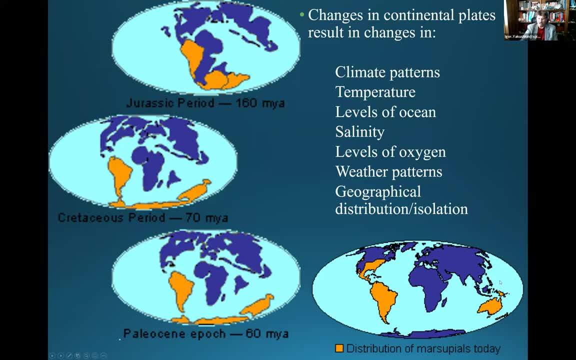 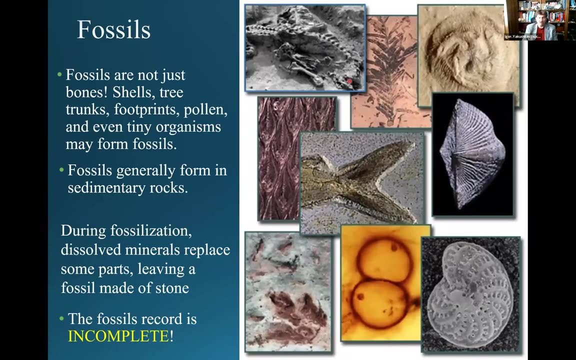 under natural circumstances outside of the australian oceania. most of it, of course, stays and you see, australia stayed quite isolated, so most of the marsupials survived there. now fossils as the evidence. we already talked about that generally for the sedimentary rock fossils are very rare, uh, very rare occurrence. so the fossil record is incomplete. why it's a rare? 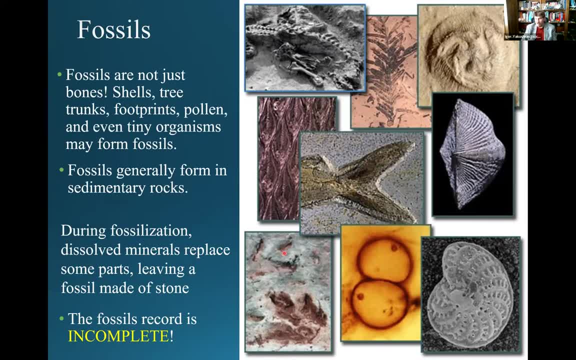 occurrence because the conditions have to be perfect. usually remember the bacteria and uh fungi are recyclers, the decomposer. so as soon as something dies, the bacteria and the fungi will start breaking it apart, unless it will end up somewhere in the deep clay, surrounded that. there is no much of the bacterial fungi there and then it might stay preserved, and i have several. 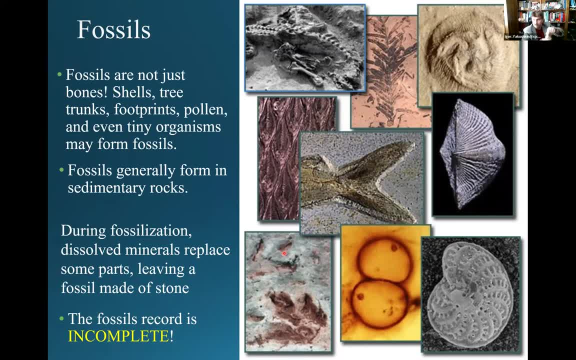 fossils. let's see, here we go and quite often, quite often, you will see that only hard uh parts of the fossil will be preserved, right, in this particular case, the shell, the soft tissues sometimes, sometimes, uh, do being preserved, sometimes not. that's the interesting one, not the rock known as a coprolite. 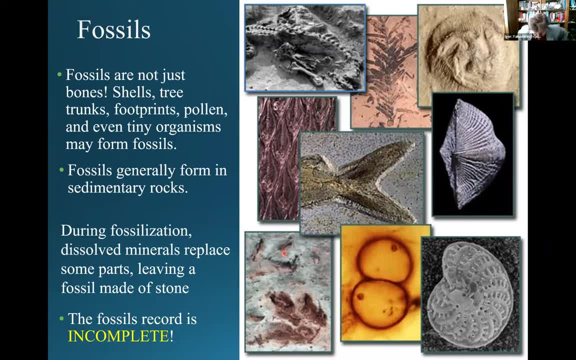 copros means feces, alitas means uh, rock, that's, the fossilized pieces, yes, so, yes, sometimes that happens as well, but in most of the cases we're looking at the hard- uh hard- parts like the, the shells, etc. and sometimes, of course, tracks will have a dinosaur tracks in texas state park, not far from. 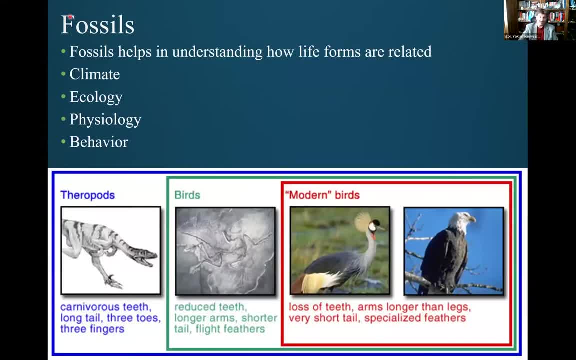 dallas. so fossils. besides, that, just we we can see that different organisms were populating the earth at some point of time helps us understand how the life forms and how they are related. we know that the modern birds are some sort of dinosaurs. they evolved from the dinosaurs. 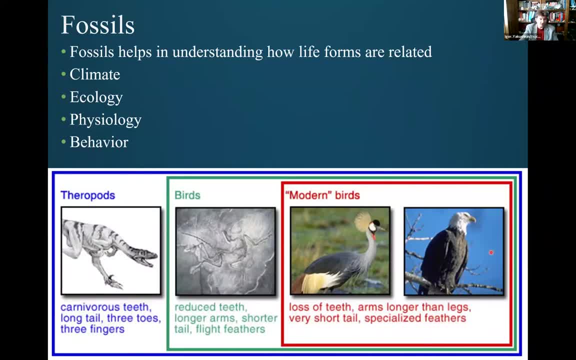 not t-rex directly, but from the same group, which, uh, t-rex belong to, as well as the girl, the lesser raptors. also, we can talk about the climate really, really well. we can say: well, the climate is why? because we know, like, uh, some of the organisms, like, for example, let's say, 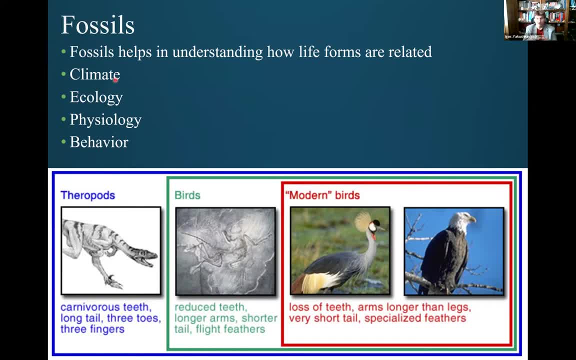 we know that at some point of time uh, antarctica was a very lush continent with, very well, a continent with a very lush uh forests. so, in this particular case, pretty much tropical forest, because we know that there is some fossils of the uh tropical plants- not anymore, but at some point of time- as as well as the uh. 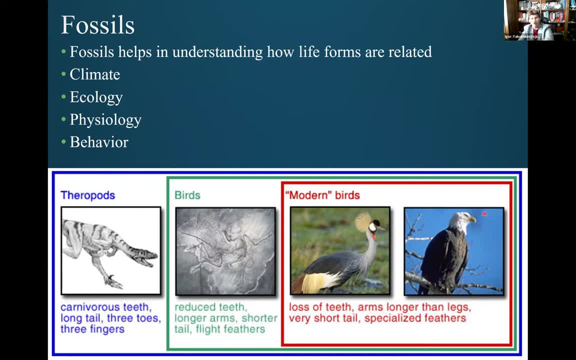 ecology and based on whatever we see in the modern creatures, we can infer the physiology as well as a little bit of uh, even a bit of a behavior, for example, let me find that particular here. oh, no, i don't should have it, no, i don't have it, uh. but right now we are thinking that some of the 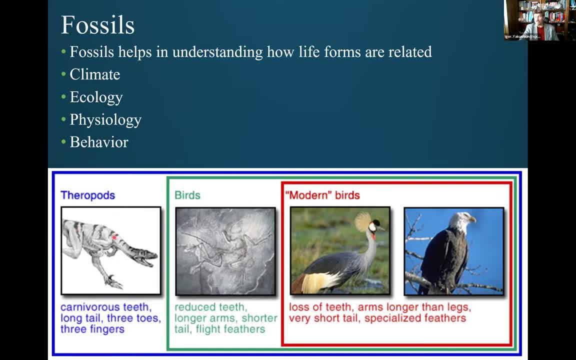 dinosaurs are most likely not all, but some of them were warm-blooded creatures. why? because of the structures of the bones. they are very similar to whatever the mammals, as well as the birds, the warm blooded creatures of modern times have. therefore, we can infer that most likely some. 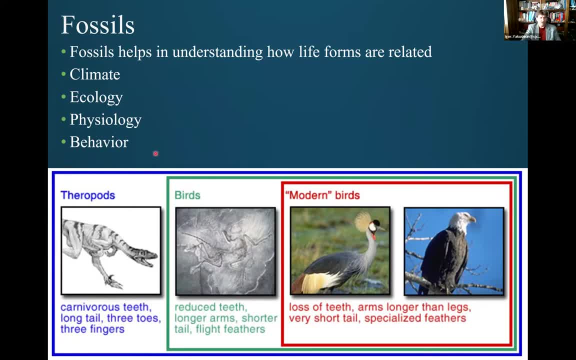 of them were uh, uh, warm-blooded creatures and, of course, based on whatever the uh, whatever we see in the fossils, we can infer as the behavior, for example, uh, dinosaurs most likely had some of the parental care, meaning that they were. they had some sort of huge nests with the eggs and then 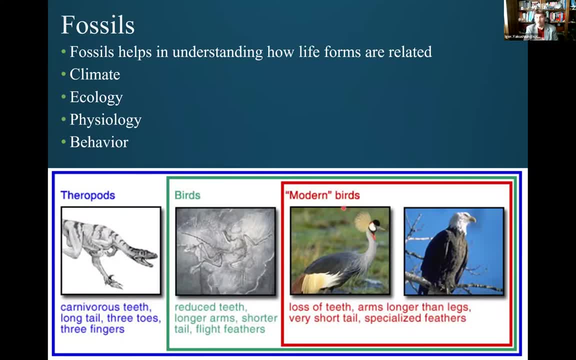 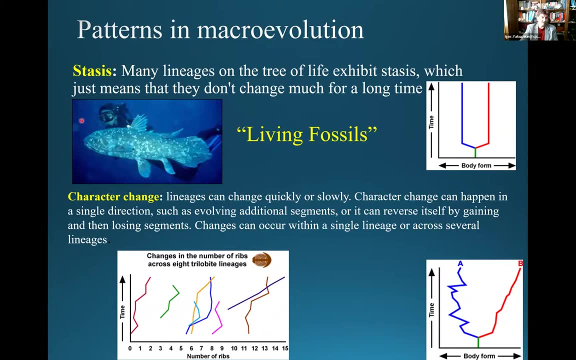 there will be a couple of adults- uh, basically protecting those nests, same idea as we have for the modern birds. now patterns, and here we have a very interesting things: stasis. stasis means that at some point of time the creature were evolving, everything was good, and then for one or another, 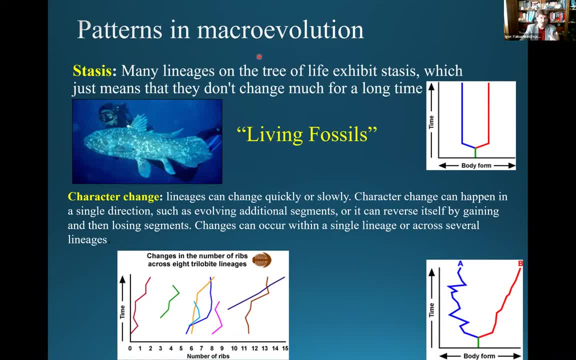 reason and we don't know a reason, and that's one of the problem with the evolution. we cannot explain it. yet the species do not change much, if at all. for example, you can see that particular weird looking fish known as the latimeria or silacan. uh, silacant was well known, uh, since 1800s. 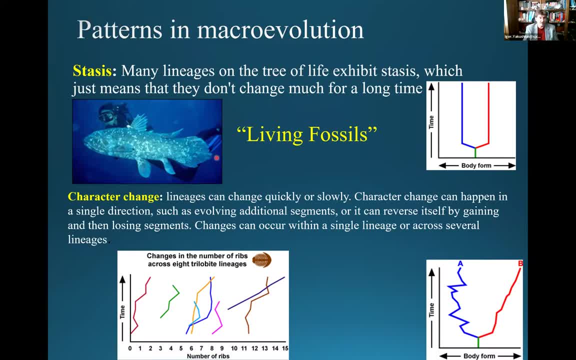 as its fossil form. it's something which known as a lobfin fish, that the group of fish most likely give us the link to the modern uh, pteropods, uh, including amphibians, reptiles and the well birds and the mammals, but in this particular case, that particular 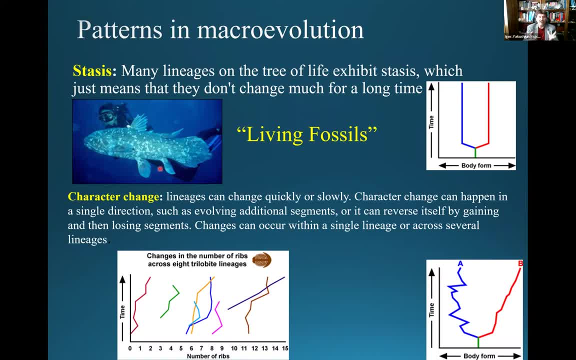 fish. we had a really good fossil record of those. and then in 1930s one of the ladies uh in the south africa- uh, the the east coast of south africa- found in the catch of the day. uh, she found the weird looking fish. unfortunately she were unable to preserve it initially, but she was able to draw out, uh well. 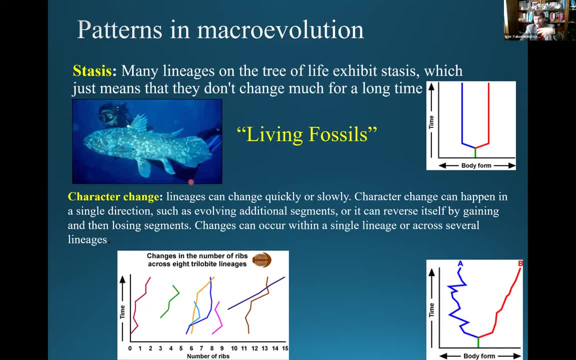 uh draw the outlines of the fish. and then she sent it via mail- a regular, not emails via mail- to her friend, like a couple of hundred miles away, who was avid technologist, and he said: you are on something, get another one. and this is uh, get another sample and this is how you need to preserve. 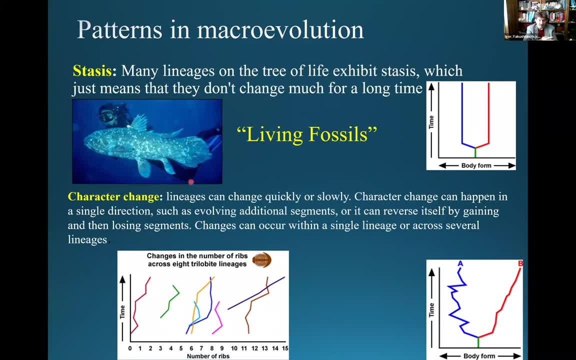 and that particular fossil at some point of time was rediscovered as the living creature. so those ones are known as the living fossils. we'll talk about those, meaning that that particular creature did not evolve for the last 300 or so millions of years- 250.. same thing with the horseshoe crab. later on we'll talk about the horseshoe crab. it did not. 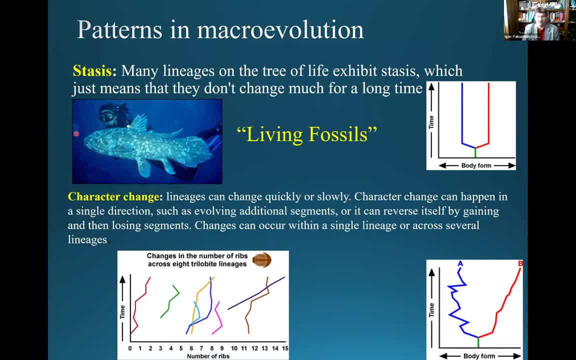 did not change much for the last 300 millions of years. why not? ah, we don't know. the climate changed, the environment changed, the horseshoe crab did not? some of the scorpions we have, the perfectly preserved in amber scorpions, and we can literally get. well, maybe not to the species. 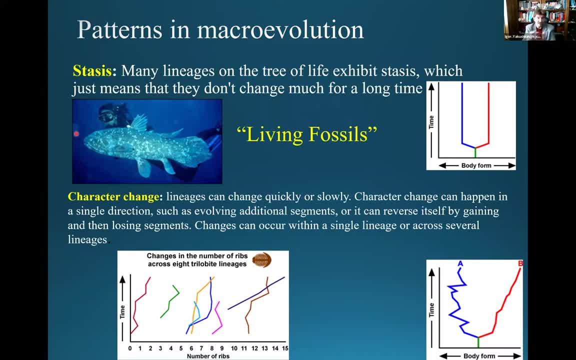 but to the genus of modern scorpions. so they did not diversify much over a long period of time. why not? well, they're living fossils now. some of the lineage will change relatively quickly. some of them will stay. uh, will stay, not change much. sharks did not change for the last 150 or so. 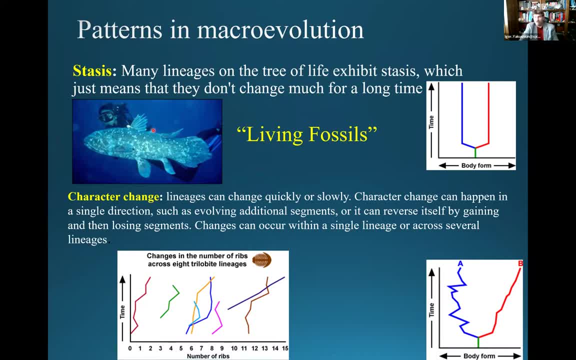 millions of years. are they super evolved? well, maybe, maybe not, but definitely could evolve a little bit better. uh, the eyesight is not the best, or anything like that, but they did not change much and once again, all of that creates a huge problem for overall evolution of theory. 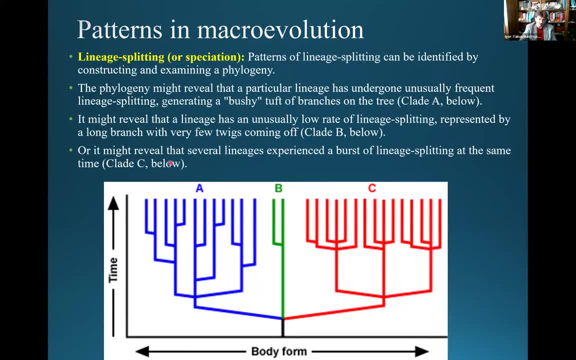 of evolution, now patterns in evolution. so some of those particular, let's say we have the art reports. we have a huge diversification among crustaceans, we have a huge diversification among the insects, but we have a very small, uh small, diversification among the silverfish. 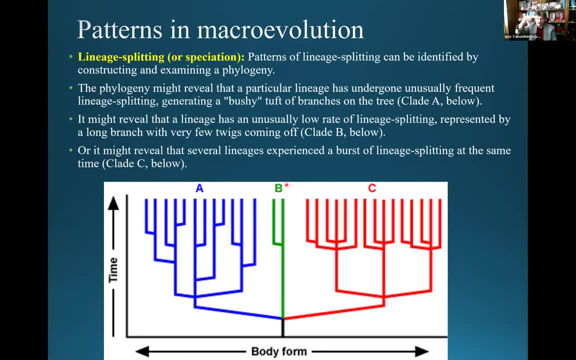 everybody's in the silverfish, right? yeah, tiny little, bitty pesky creatures right running around. so those ones we're looking at, about 500 species whenever the insects are in millions, why some of the groups stay, uh, within a handful, so to speak, of species. another one: 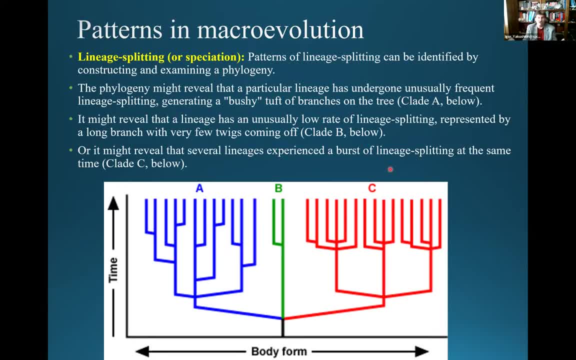 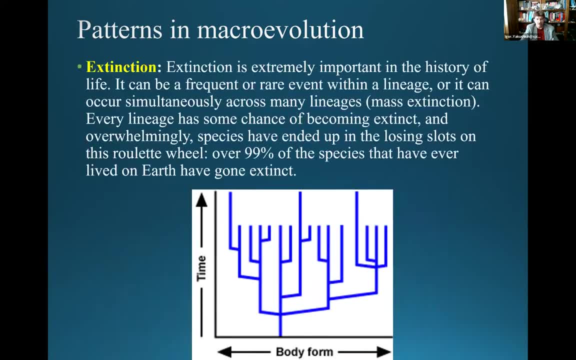 went and diversified into a million, we don't know, cannot explain per se. then of course we can go and look at the extinction. extinction is important, mass extinction specifically. so you can see, at this particular time bunch of different groups extinct, cease to exist, some of them to continue. 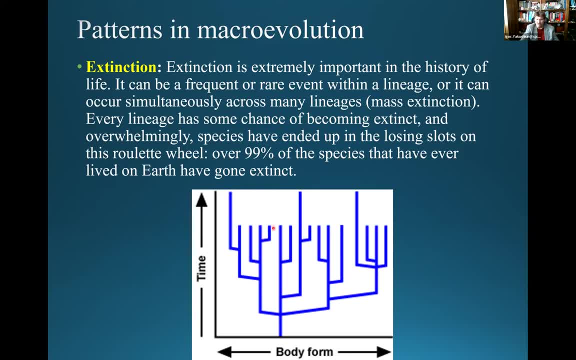 but many of the groups still exist. think about 65 millions of years ago. a lot of dinosaurs and other creatures died off. some of them survived and now we call them birds, right? crocodiles survive- some crocodiles died off- many of them- and alligators survived. rep uh, the lizards and the snakes. 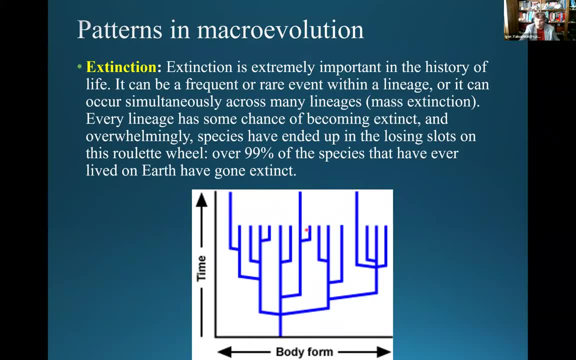 survived. they were, but some of them did not. uh, dinosaurs did not. so in this particular case, this is the mass extinction. what's really happening? you can say: well, the best extinction is bad. yes, mass extinction is drastically reducing biodiversity initially, but often, often, what we see after the mass extinction, we have that particular line and then it's bursting into. 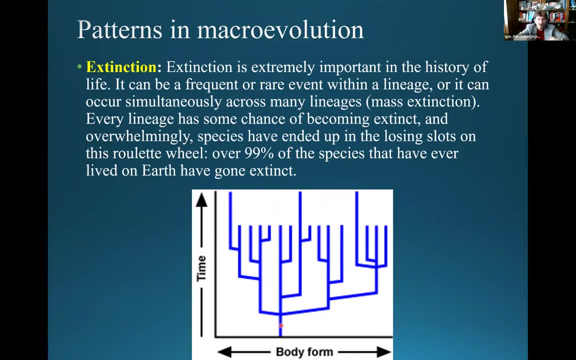 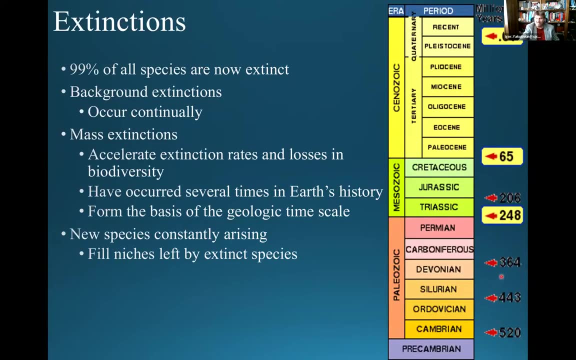 a diversification. so after the mass extinction we usually have the uh boost in the biodiversity and this is how essentially, let's say, mammals uh being diversified, and i'll show you the example of that. so there is a several major mass extinctions. we have one, two, three, four, five, six. 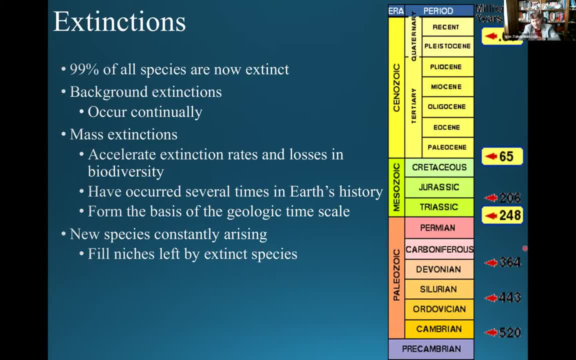 six, six. well, uh, well documented. there was a smaller extinction between those, the permanent extinction. i already told you that was one of the bad ones, 65 millions of years ago. uh, the extinction killed pretty much most of the dinosaurs and other creatures, uh, some of the mollusks, etc. and now there is a possibility that we're living. 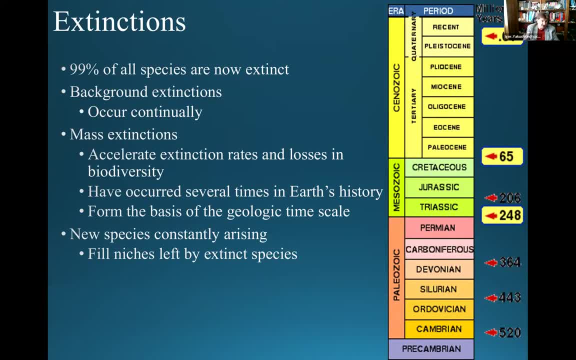 in something which known as the seventh mass extinction system. so we just have the uh, uh, uh during the uh explosion or uh eruption of that particular super volcano in siberia. by the way, well, whatever is, it wasn't siberia back then. it's now central part of siberia. uh, the city of perm, you can look it up. so, anyway, accelerate. 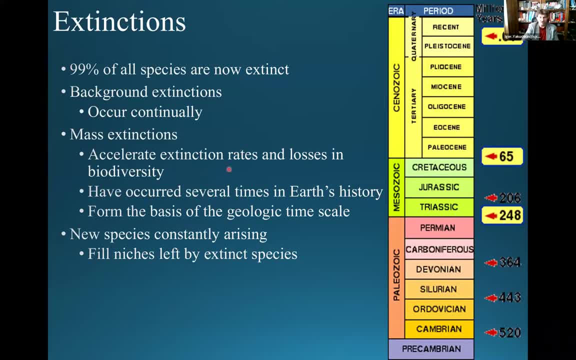 extinction rates, meaning that the species are dying off really, really fast. but if you look right here, 99- basically 0.9- of all of the species which ever been on this particular planet already extinct. so whenever you will find any kind of person for saying we are so horrible to the 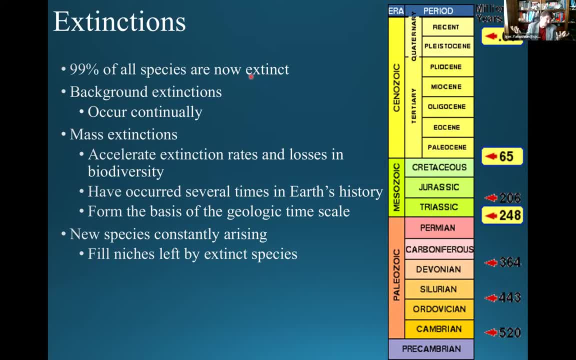 mother earth and we're killing the species, etc. etc. you can say: well, maybe we're just helping the mother earth because 99 of the species already extinct, we're just helping to speed it up, those particular species which we don't like, or maybe they're not very well adapted- cockroaches, all. 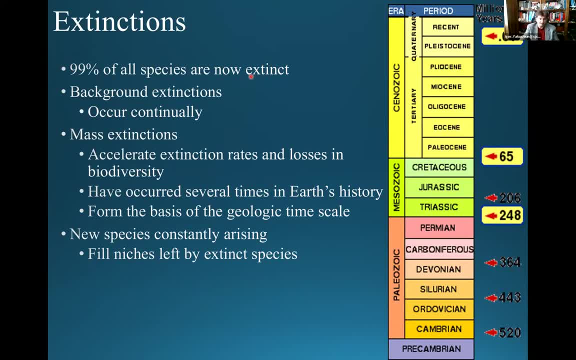 over the world. tigers not so much, you right. so anyway, what's really important? that usually after the mass extinction, new species are constantly uh arising and because we start seeing the available niches, roles in the environment, we'll start seeing the burst in the uh, in the diversity. 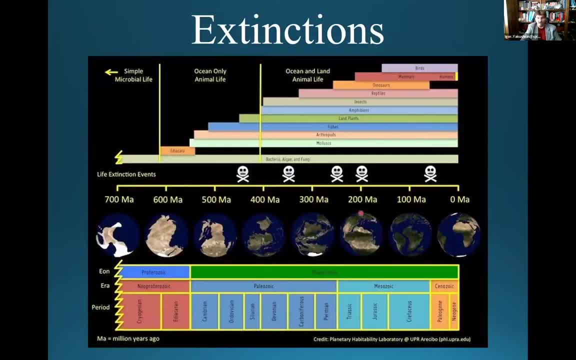 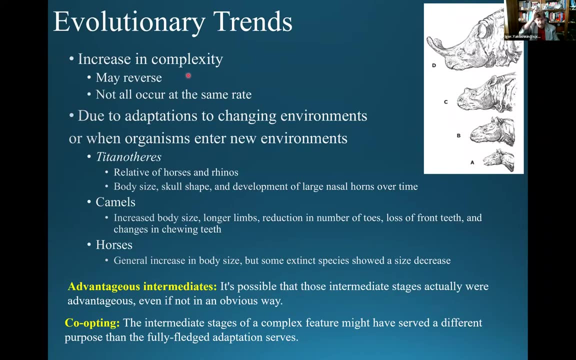 after the mass extinction. so this is one of the major mass extinctions and we might talking about the red on the bottom left, the mass extinction in the san angry extinction right now nowadays, so to speak. so another some of the evolutionary trend increase in complexity. that's a general idea, uh, starting. 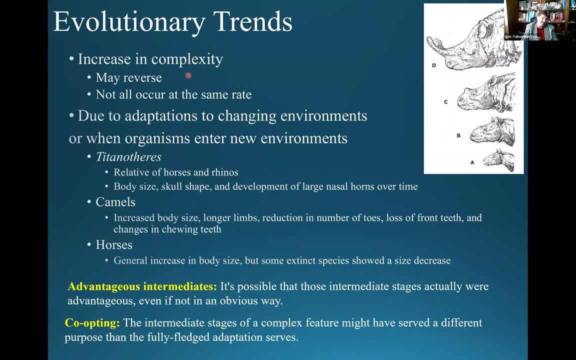 with lamarck that every amoeba is on the way to the human uh being. not necessarily. we have a whole bunch of parasites which usually are simplifying the uh uh, the, the body, uh body plant like uh a of the viruses. how the viruses started. there is idea that viruses initially were parasitic cells. 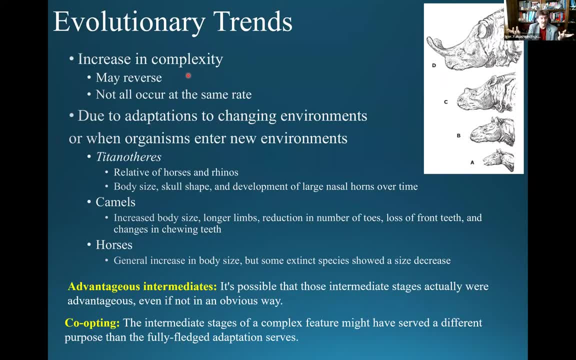 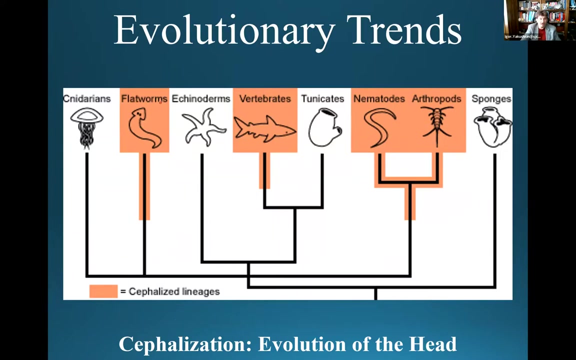 which lost most of the cell components except essentially dna. so increase in complexity sometimes happens, in some cases it doesn't. and then of course we are talking about the um, the evolutionary trends like, for example, cephalization, cephalos- cephalos means head, head. uh, the flatworms come up with that idea, but they come up on it separately from us, the 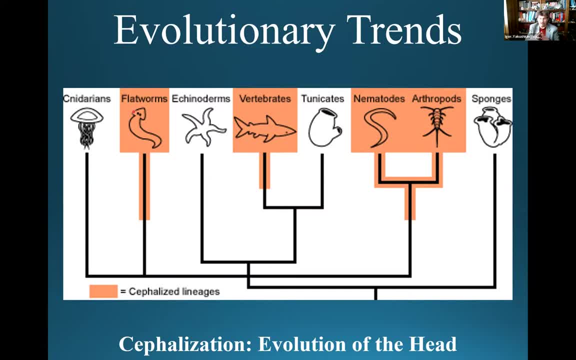 vertebrates. what is head essentially is- and please make sure you understand that head is the front end of the body, which goes and starts sensing the environment as a result. as a result, the front end typically carries a lot of sensory organs: the pressure touch, the chemical smell and taste. 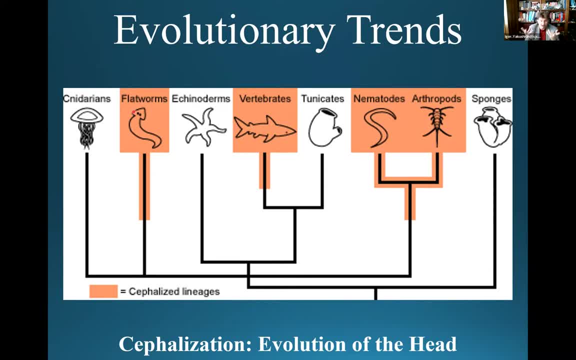 the, the uh light sensors, the eyes and so on, so forth. but that's the only part of the deal. another part of the deal: if you have all of those sensors sending all of that information, you have to have the uh, some sort of processing unit, brain which will process. 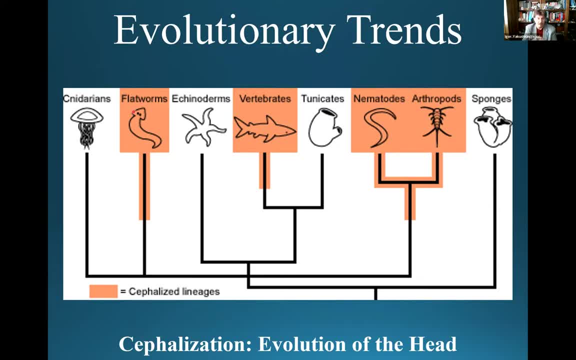 and react accordingly from those particular, from those particular sensory signals that we're getting, or the the creatures are getting. so it goes in the in kind of correlation. we start seeing the increase of the sensors, complexity of the sensors, we'll start seeing increase in complexity of the brain and the brain will be moved toward the forward part of the body. 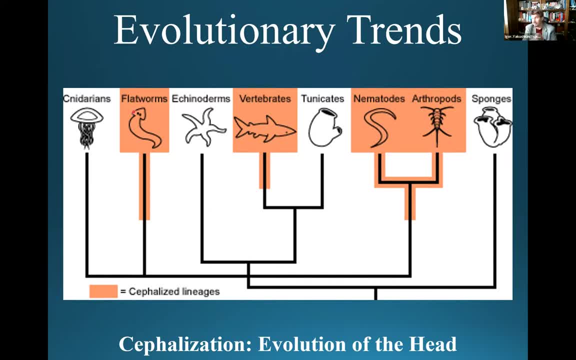 why, in order to send the signals pretty much, or receive the signals almost right away, we still have the- uh, slight bit of the brain that is moving towards the forward part of the body. um, but in our case, we're seeing a delay from whatever we're seeing. it's like 0.8 milliseconds. 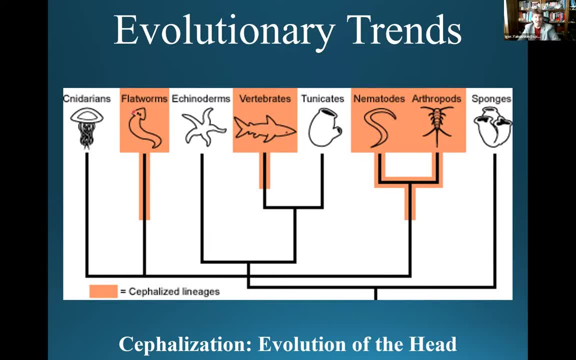 so whatever you see is already happening 0.8 milliseconds away, uh, uh ago, because once again, the our eyes sending the images to the brain, brain have to interpret. all of that takes time. so we live in a essentially path, but it's it's a very, very narrow. so, as you can see in this, 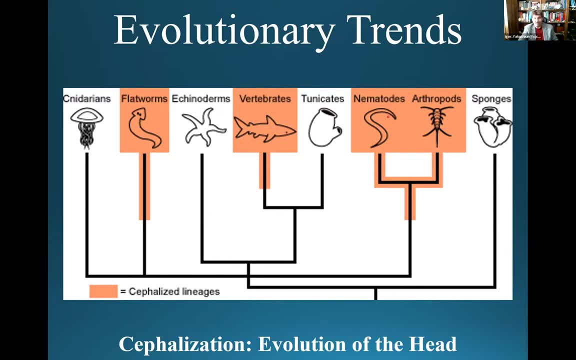 particular case, the civilization is not so much about the brain as it is about the brain and the. the formation of head happened in the different groups, essentially separate nematodes, which is the round worms, and the arthropods. they had the common ancestor and most likely they had started. 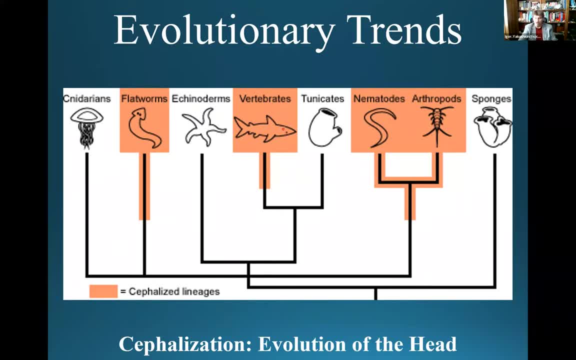 to get well, started right here. and then they split, but vertebrates not exactly. we're starting with the tunicates, which is which does not have head but well, as an adult, they have it as the larvae, and this is where the cephalization, so the process of cephalization, happened in the 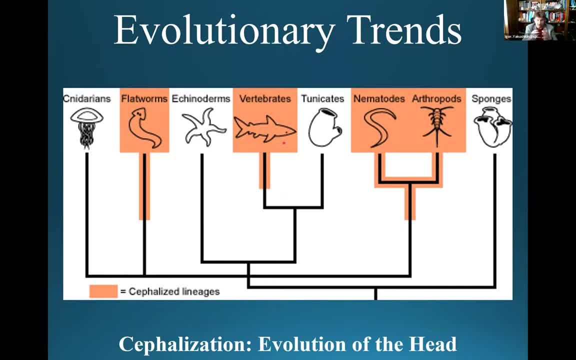 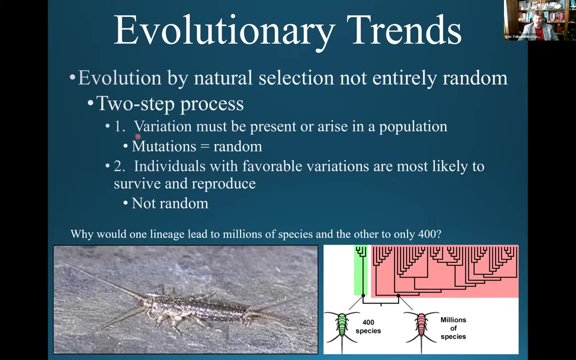 different lineages at a different time, but again, it's all based on what the which end goes into the environment. same same problem, solved essentially the same way. so, moving on almost over so evolutionary trend, we'll talk about the two step process. variation have to be, so mutations are random and then favorable variation will be. 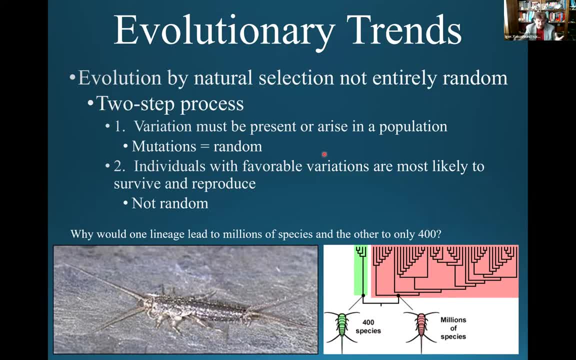 selected by the nature right natural selection. that one is non-random. mutations are essentially random mistakes in the dna. that particular mistake might give you some sort of positive input and this is the favorable variation, typically 99.999. one out of 10 000 mutations are beneficial under these particular circumstances: 9999 of them. 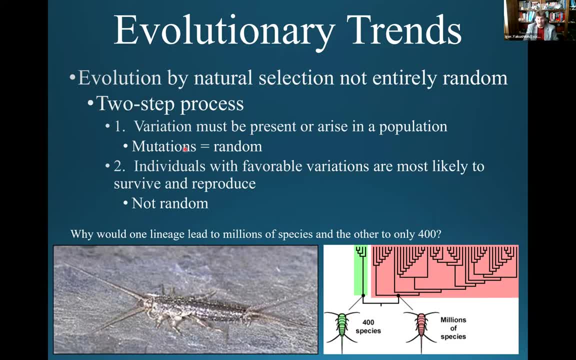 will either have no effect on the organism or will have a negative effect on our organisms. so once again, we have, in this particular case, natural selection works on two steps: random and then the preferential non-random. and we already talked about the silver fish- silver fish within the 500 species, or 400 species- and the millions of insects, even though they started. 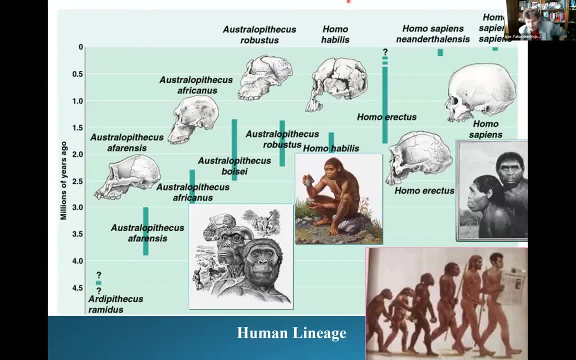 with the same ancestor and we already talked about the another example of the process of evolution, starting with some sort of australopithecus through the time getting into your homo sapiens. you don't really remember how to spell australopithecus, you can say ancient hominid. 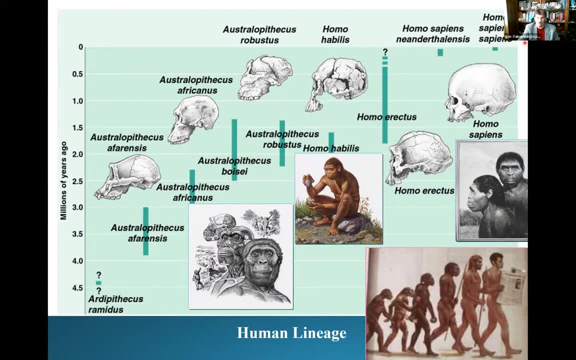 into your modern human all right, or homo erectus, gradually evolving, not directly, it's not like homo erectus. and then we have the homo sapiens. no, there was quite a few different species in between, but from homo erectus into your homo sapiens, that's the process. 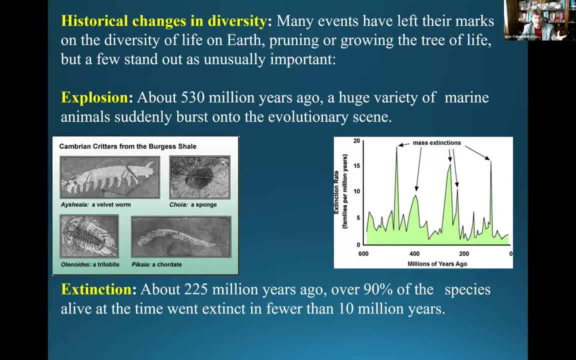 all right, change in diversity. we already talked a little bit about that- the extinction- and then we're looking at the uh, at usually we start looking at the uh- increasing of the biodiversity- already talked about. 225 millions of years ago we had one of the major mass extinctions. 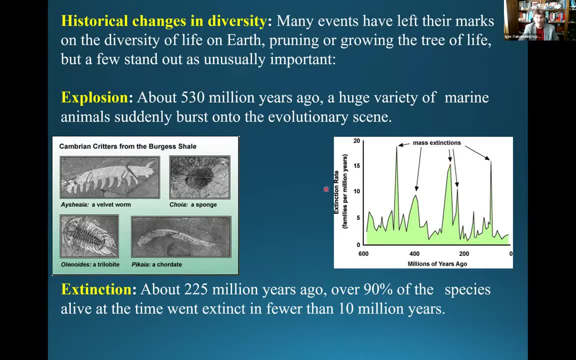 which basically known as a permian extinction, and in this particular case, uh, lots and lots of creatures died off, and you probably uh heard about the burgess shale. it's, it's, uh, it's basically a clone diet. well, it's not clone that per se. it's, it's, it's a holy grail of the paleontologists because 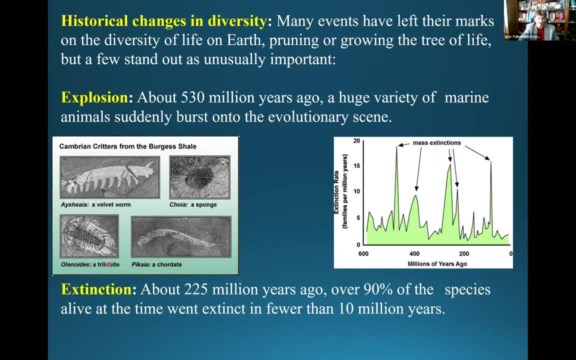 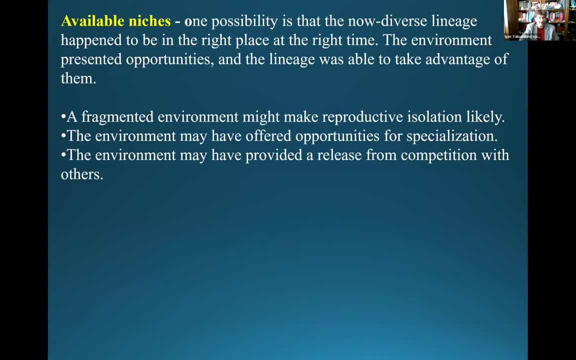 you can, uh, you can link quite a few creatures, uh, from there, and it's about 530 millions of years. all so available, niches, again, availability to do something on the scene in the nature and a theater of the nature. now, once again, remember, no two actors can occupy no two species. 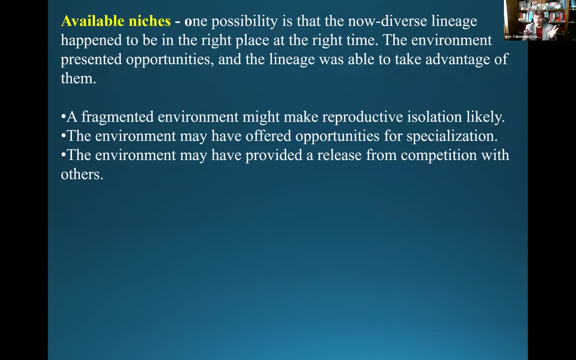 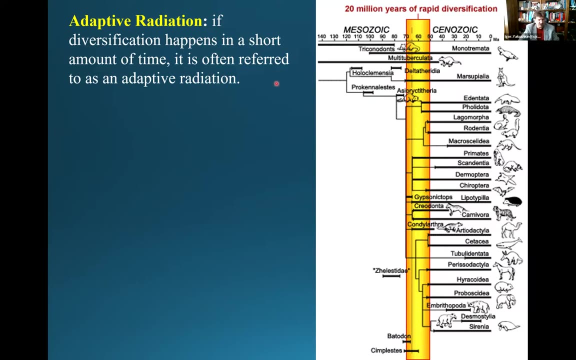 can occupy the same role. parallel, yes, similar, yes, but they're the same. they start inter-competing and then one of them have to perish or switch to something else. so, and here we're looking at the adaptive radiation. look, uh, mammals evolved around 200 million of years ago. uh, but by that? 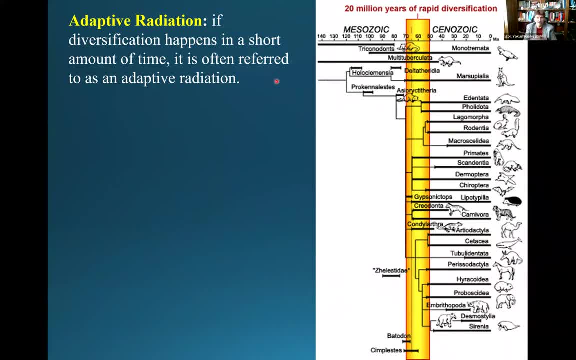 time the animal. they evolved every year. so they got phase despair because at the center of the god evolved we start seeing we essentially the dinosaurs were already in the full swing to take over the planet. they took over the planet and they had it for almost 150 millions of years. 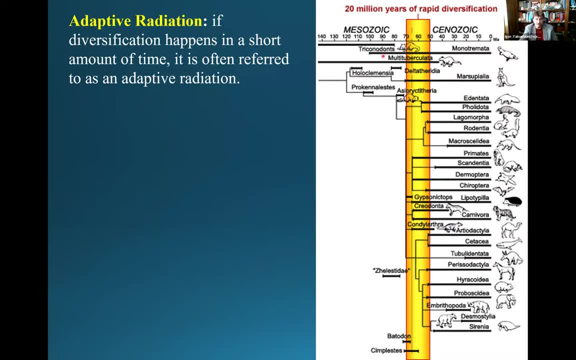 until 65, and our ancestors, uh, rat looking creatures or opossum looking creatures- not the opossums we know right now, but opossum looking creatures- relatively small, mostly nocturnal creatures- lived in the literally shadow of the dinosaurs. dinosaurs didn't give the. 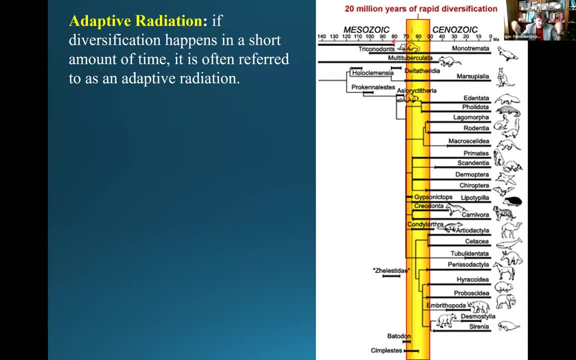 chance to the mammals uh to uh proliferate, to buy the oil. to diversify: why not? well, because there was no available niches, one of the most common niches. as you know, most of the reptiles are not active during the night, so the mammals become active during the night. 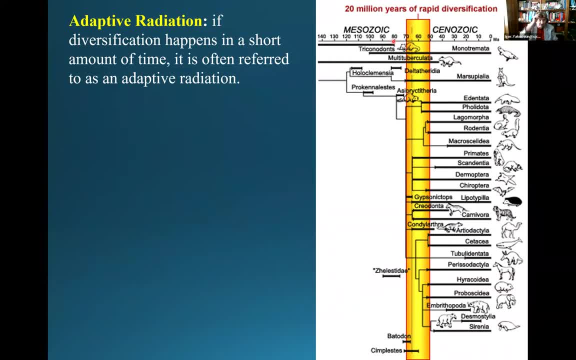 which play the very important role: information of the mammal brain. why think about it during the night? you have to have much higher senses, right? you have to smell better. you can have here better. there is not much light, so you have to have a better vision. all of that you'll have to have. 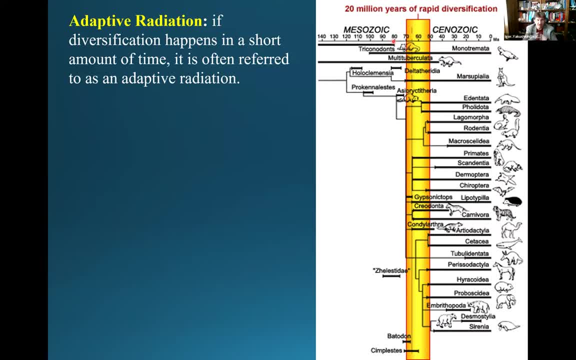 more acute senses. more acute senses will require a bigger brain to process all of that information. bigger brain, so the mammals become brainiacs of their time. but again, the dinosaurs were happily jumping on the uh on our ancestors until 65 millions of years ago. something happened. 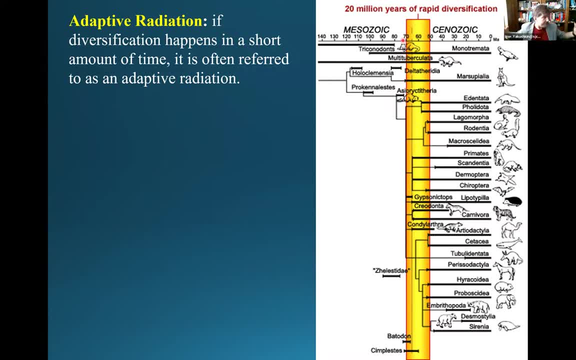 most of the dinosaurs wiped off, and then the mammals, like nobody is eating us. and then, look, we start seeing huge diversification of the mammals. literally after this is the mass extinction of the dinosaurs and a few other creatures, or quite a few other creatures, and then in the next 15 or so millions of years, we start seeing the marsupials. 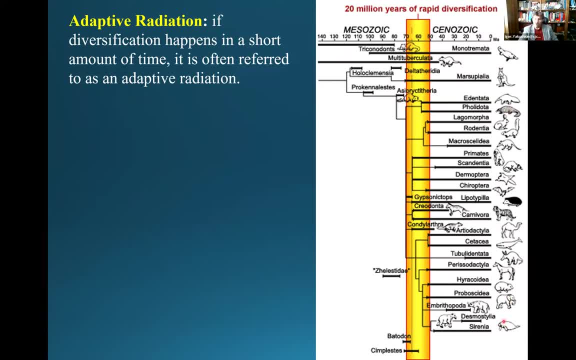 marsupials, as well as the monotroms and pretty much all of the groups of the modern mammals. the primates come out, the rodents come out, the uh primitive hairs come out, as well as the red uh rabbits. the carnivores showed up, and so on, so forth. so there was not that much of the diversification when the